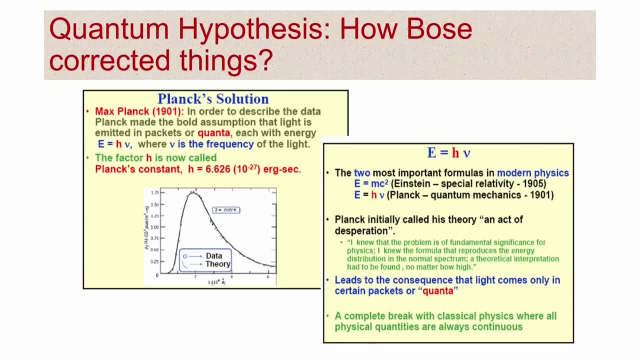 discussion on the emission of electromagnetic radiation as a function of temperature. You must have seen that when piece of iron or a metal is heated, it initially becomes red hot and then it becomes white hot, and so on. So the spectrum of the incident radiation changes the frequency of wavelength from one 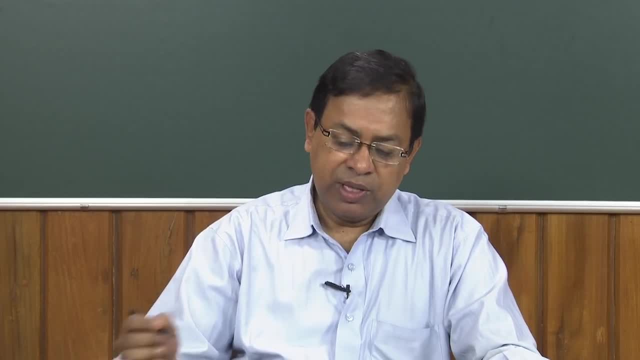 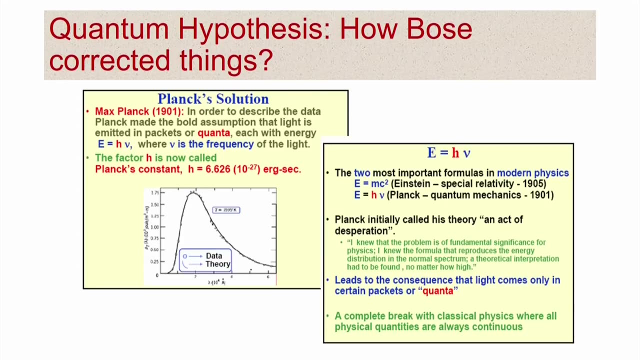 to another and experimentally it is found that the spectrum, the incident radiation intensity of the radiation versus The radiation intensity of this radiation versus this wavelength in respect in value, theелk. 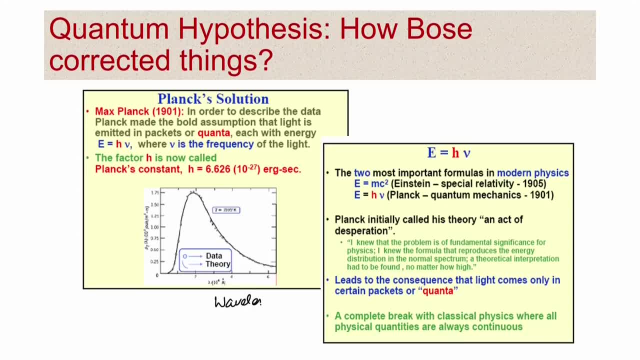 wavelength. So this is the wavelength. if you cannot see it, these are on small fonts and this is the intensity. So that looks like this, However. so there is a non-monotonicity at a given value of the wavelength and this was discovered experimentally and the classical 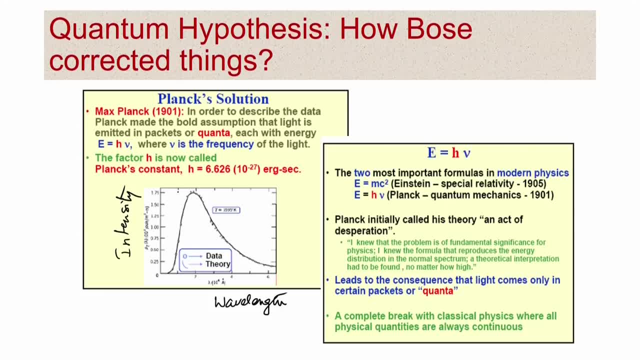 existing classical theories predicted that either it is like this or it is like this, which are according to the Vien's displacement law or and the religion's law. However, this non-monotonicity nobody got theoretically. So Bose understood that there are rather 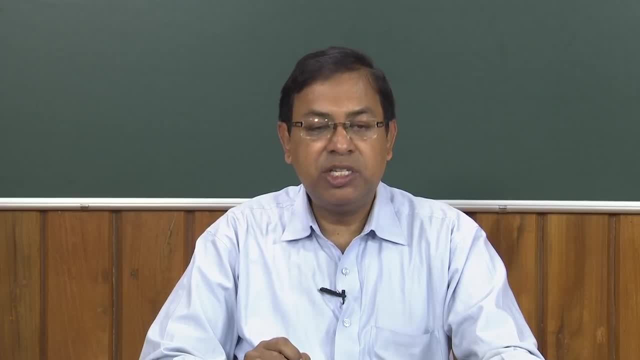 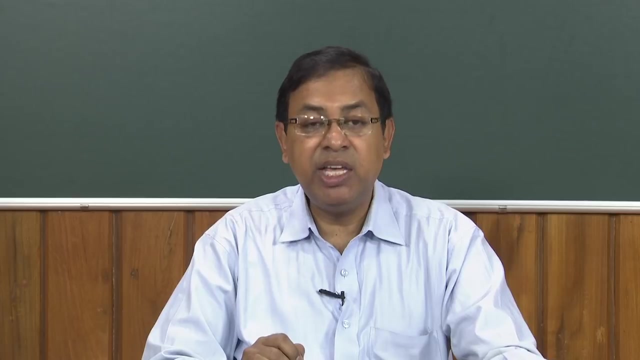 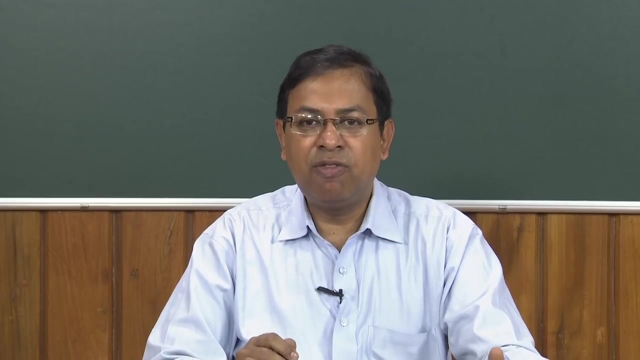 in fact, Planck proposed with just conviction and no sort of conviction Theoretical backing. however, Bose said that there has to be a new statistics for the photons or the incident or the emitted radiation, and this laid the Bose Einstein statistics to be proposed, which he did in consultation with Einstein and with help from Einstein. So 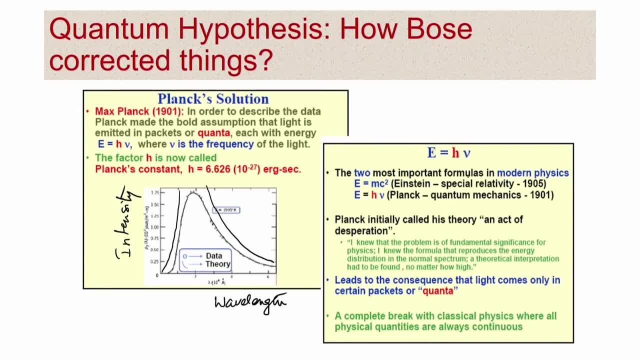 it said that the emitted radiation. Radiation has an energy dependence which goes as h nu or in quantum of h nu, and this was a birth of quantum mechanics. in some sense, However, the statistics governing this- photons are the statistics is given by the Bose Einstein distribution. So let us look at how the condensation 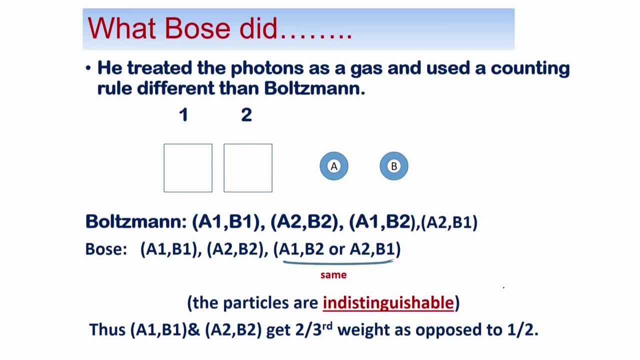 phenomena come into the picture. So let us say that there are indistinguishable particles, So bosons are indistinguishable particles, So bosons. photons are bosons, phonons are bosons, So they are indistinguishable. 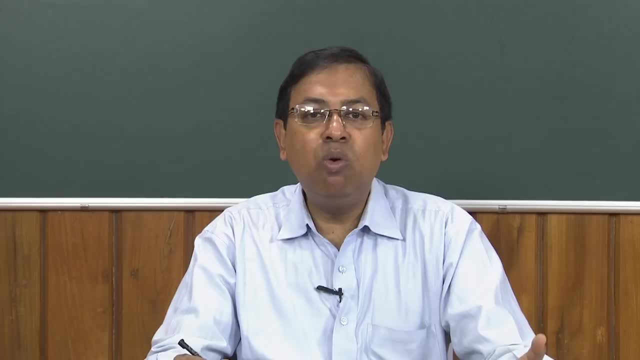 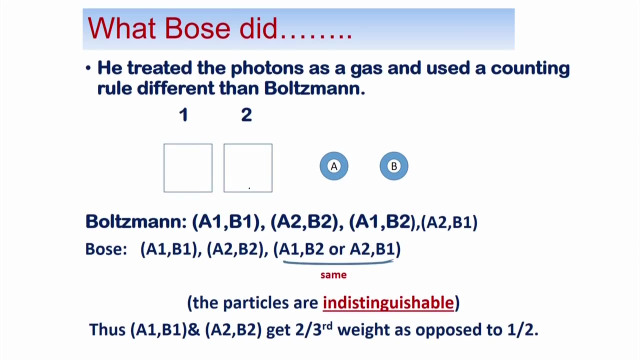 and let us see that how a simple counting procedure can give rise to a condensation like phenomena. So let us take two boxes and two balls marked by as a and b here, And let us consider them as classical particle or Maxwell-Bolzmann particles. So the particles 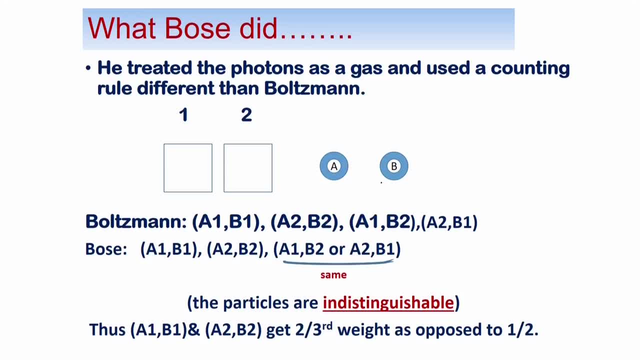 over Maxwell-Bolzmann statistics, which means that they are distinguishable. So if they are Bolzmann particles, then we can have a to be in one. So the first one refers to the particle nomenclature or the name of the particle, and one is the corresponding to the. 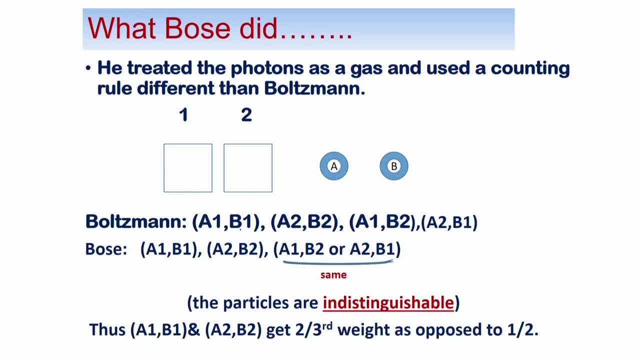 box index. So a could be in one, b could be in one as well, because there is no particular, there is no restriction on the number of particles to be occupying any quantum state, or it could be that a could be in two, b could be in two, or it could be that a could be in. 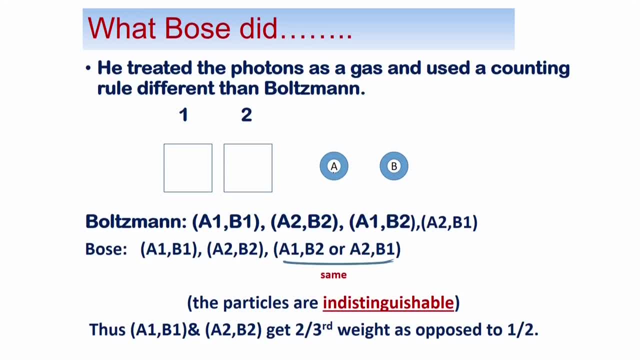 one and b could be in two, or it could be that a could be in two and b could be in one. So there are four possibilities and if you look at this, four possibilities there are. these two possibilities are that they are together, These are bunched up in the same box, So there are two out of four is the possibility. 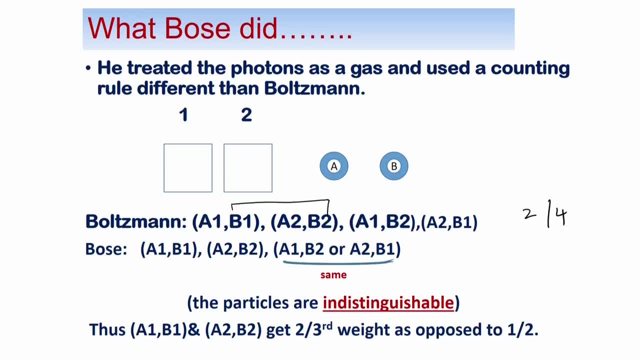 of them being together for a classical particle, or set of classical particles, which are represented by the Maxwell-Bolzmann statistics, which means they are distinguishable. Now, coming to the Bose particles, which are indistinguishable we could have. there is no, now no difference. 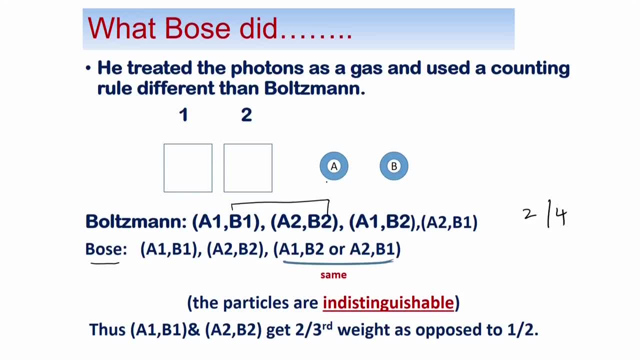 between a and b, just for our reference that we have written as A and B, but they are just both of them to be, say, A. So both of them to be in box 1 is one possibility because the bosons do not have that restriction of occupying the same quantum state as the fermions Fermions 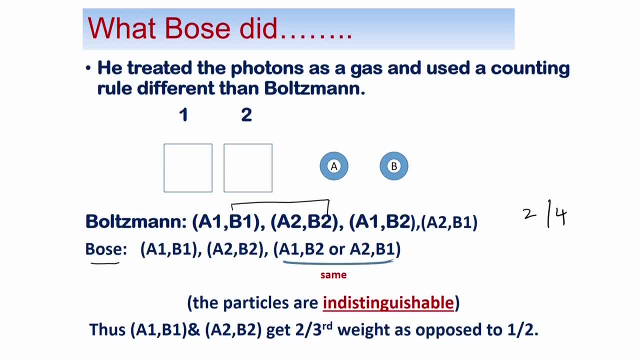 obey exclusion principle, which we have said a number of times during the course of this particular advanced condensed matter, physics. And then both of them could be in the second box. remember, these nomenclatures are just hypothetical in the sense, for our own convenience. they are both A's, So both of them are in A 1, both of them are in 2, or both one is. 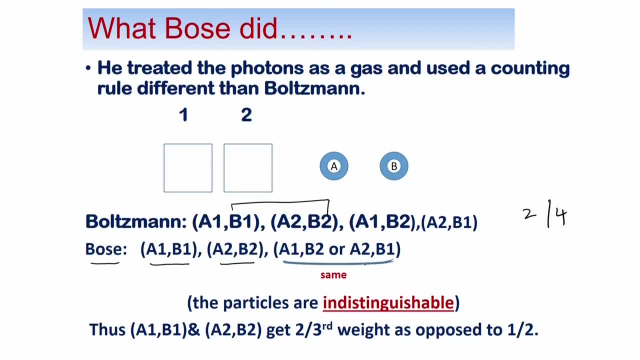 in 1, the other is in 2, or the reverse happens. So now if you look at The bunching probability, then you will see that 2 out of 3 are bunched in the same quantum state. and so this is the crux of Bose-Einstein condensation, that the statistics says, that 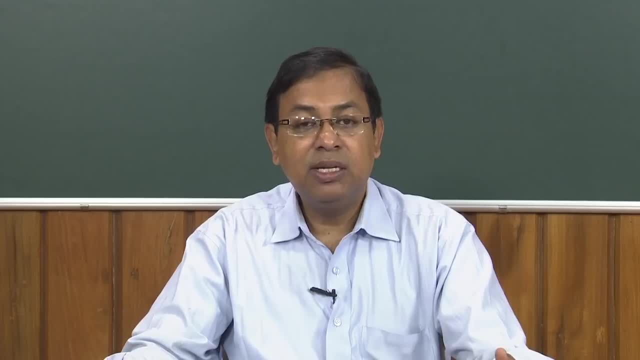 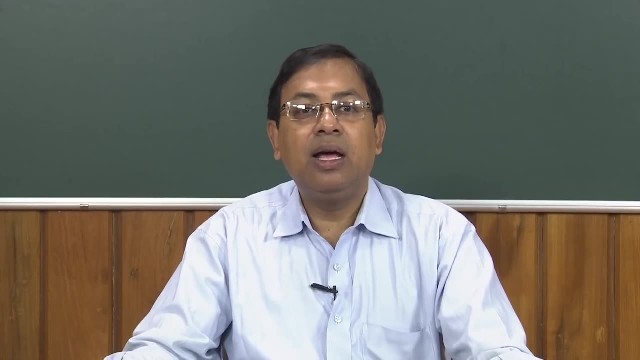 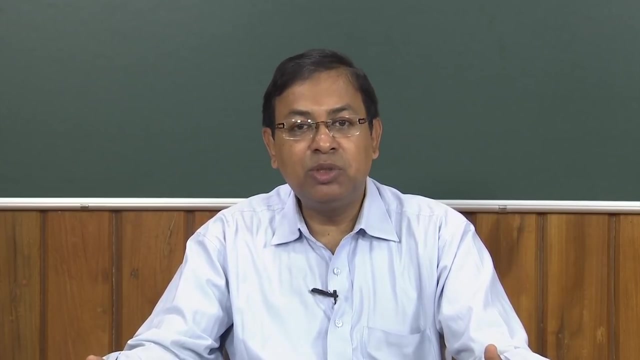 if the number of particles, that is the large number of particles, can actually occupy one given quantum state, then they will bunch up, or rather they will occupy, occupy, crowd in that quantum state and that quantum state at very low temperature would be the ground state of the system. So a macroscopic accumulation of particles in the ground state. 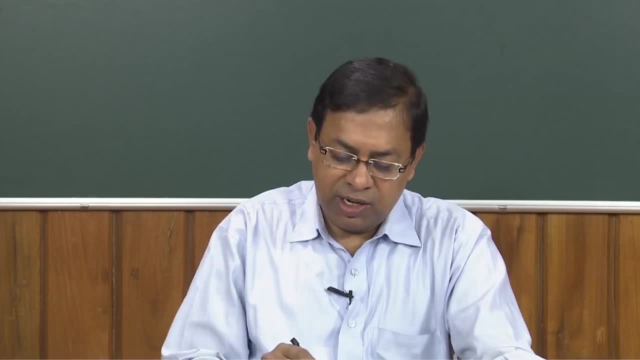 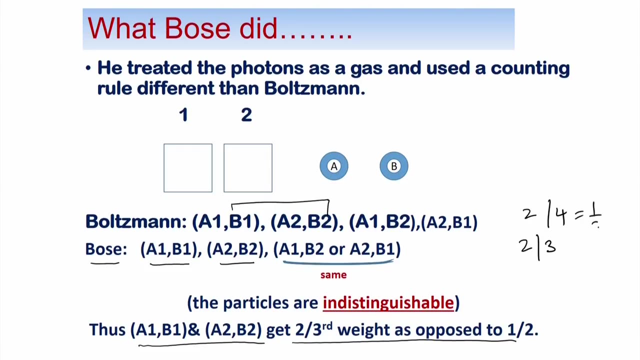 is what is known as the Bose-Einstein condensation. So this is what is written: that a 1, b 1 and a 2- b 2 get two-third of the weight as opposed to half. So this is equal to half, which is: 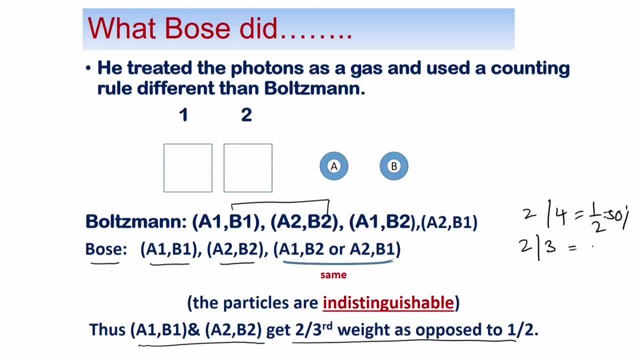 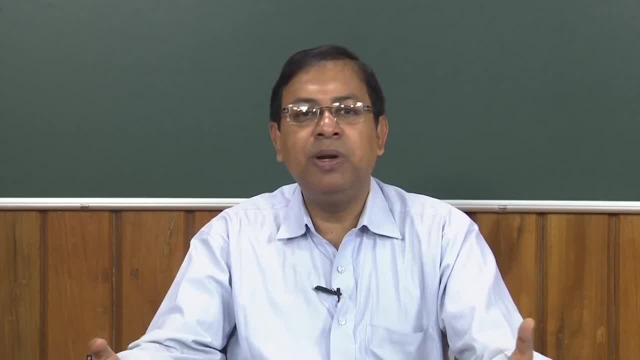 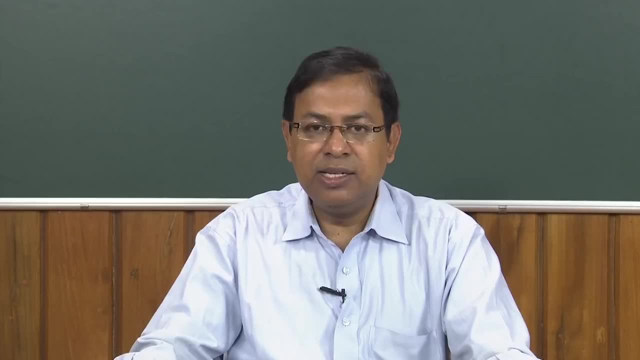 50 percent, and this is two-third is equal to 67 percent. So there is a larger possibility- and this could actually happen in a many particle sector- for us to understand Bose-Einstein condensation. Of course we are going to go details into that, but this is a very simple. 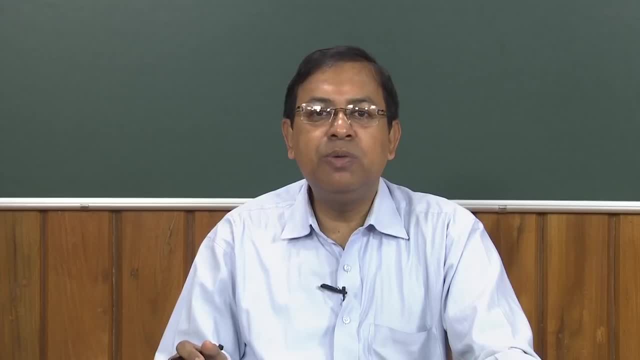 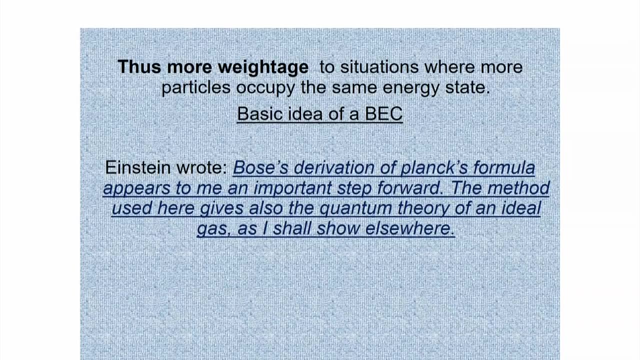 idea, summarizing that how indistinguishability of particles can lead to a condensation phenomena. So the more weightage to situations where particles occupy the same energy state is the central idea, or the central focus, basic idea of a BEC. And so Einstein, upon receiving a note from S N Bose, he understood that there is a lot. 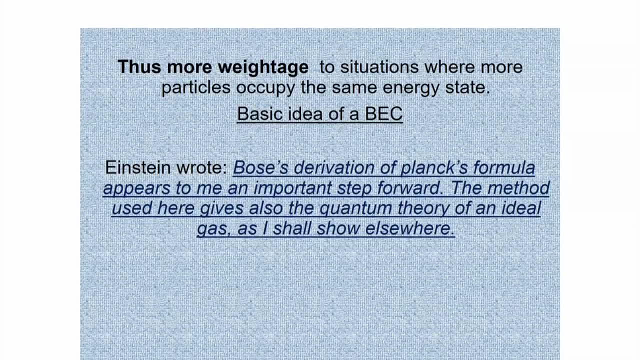 of merit in Bose's derivation of the Planck's formula, and he says that Bose's derivation of the Planck's formula appears to me an important step forward and the method used here gives also the quantum theory of an ideal gas, as I shall show somewhere. 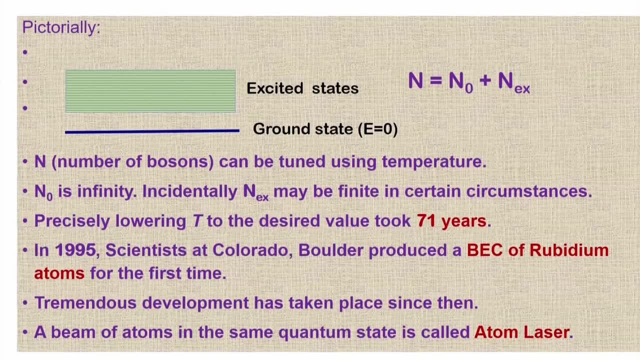 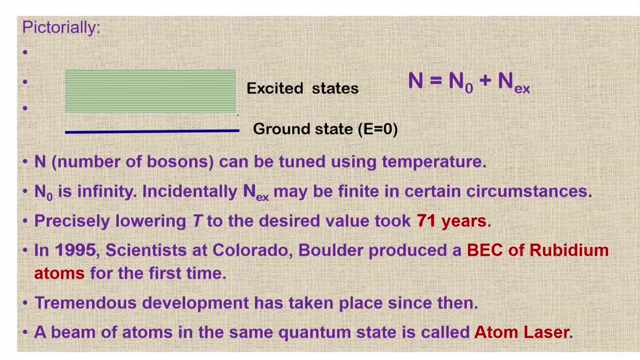 So, pictorially, let us see what happens. So there are. there is a ground state of a system which corresponds to E equal to 0, and these are the spectrum of the quantum, of the excited states, and we have just shown them almost like a continuous spectrum, because in an infinite 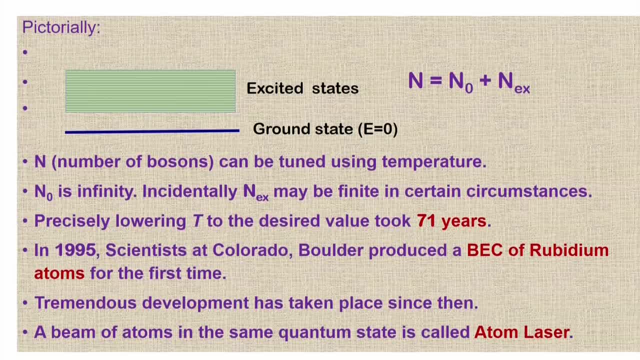 system or a thermodynamic system, they could be infinitesimally close to each other. The reason that we have shown the ground state to be separate from the excited state is something that I am going to discuss later. because of the density of states going as a particular 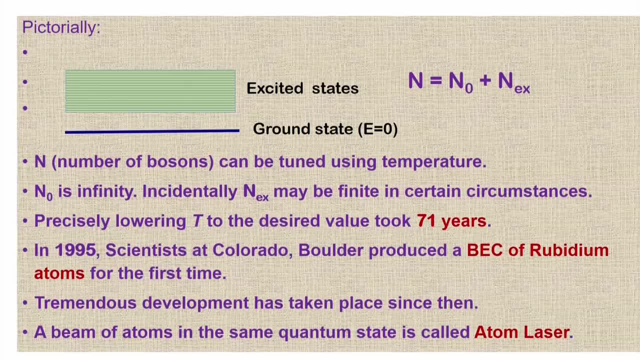 fashion as a function of E, which is E to the power half or square root of E. This is getting 0 weight, which it should not be 0 weight. So it should not be 0 weight. it should not be 0 weight. it should not. So, a priori, you cannot assign a 0 weight to any given. 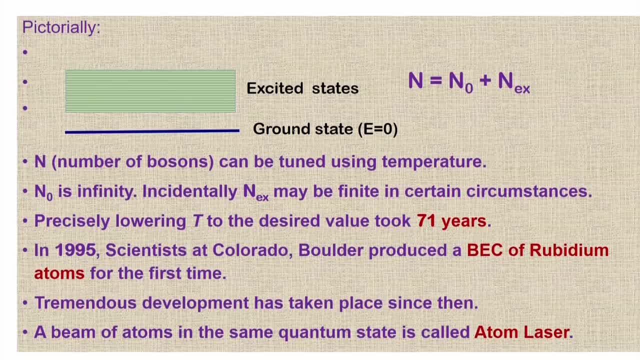 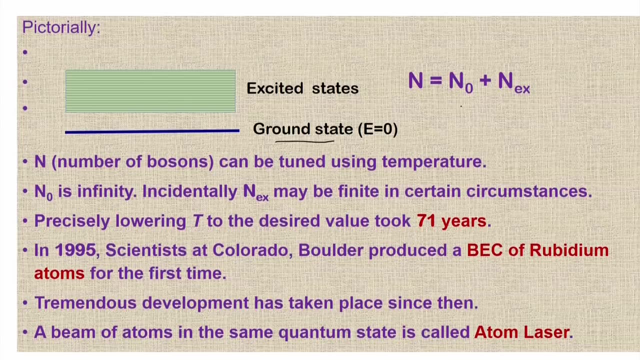 quantum state. So we are going to consider this ground state separately as compared to the other excited state. Now see, say there are n particles, n bosons in a given system where n 0 would occupy the ground state. just to let you know that the ground state has. 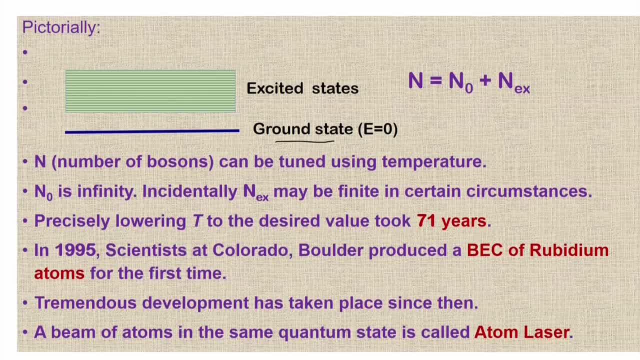 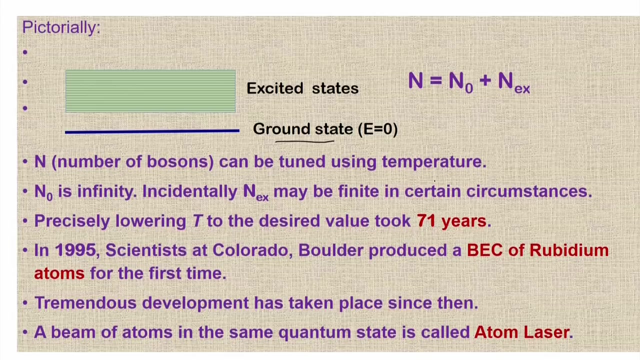 in principle, infinite occupancy will show that at lower temperature. and n E x is the number of particles occupying all the excited states put together. So now the number of bosons n can actually be tuned using temperature. It is a function of temperature which comes out of the Bose distribution function. Now n 0 is, as I said, 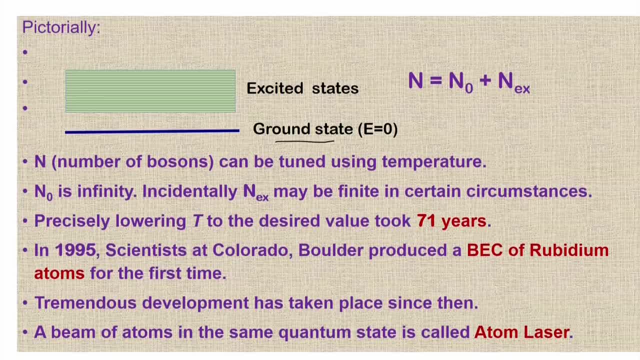 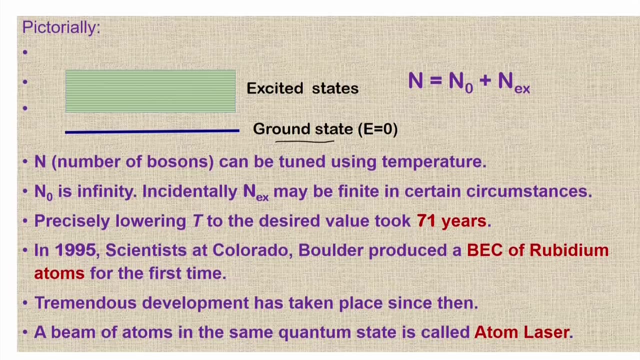 at very low temperatures, is practically infinite. Now, incidentally, depending on certain conditions- and I will also speak about those conditions- n E x may be finite in certain circumstances And, in fact, to get n E x to be- rather to get n 0 to be- infinity, you need to go to very 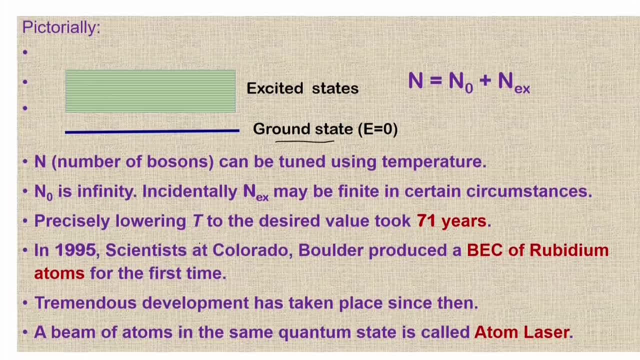 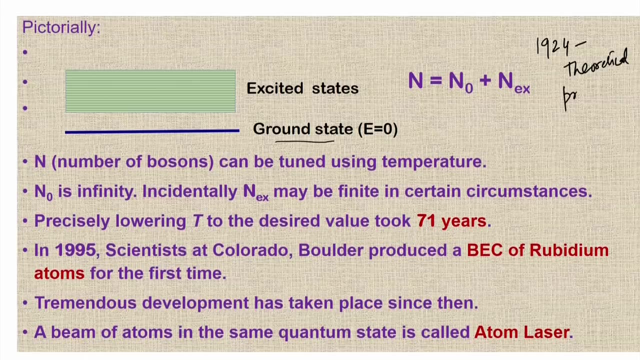 low temperature And precisely lowering that temperature, lowering t to the desired value, to 71 years. I will tell you why it is 71 years, because 1924 was the theoretical prediction of BEC by Bose and Einstein And it was 1995, as written here. 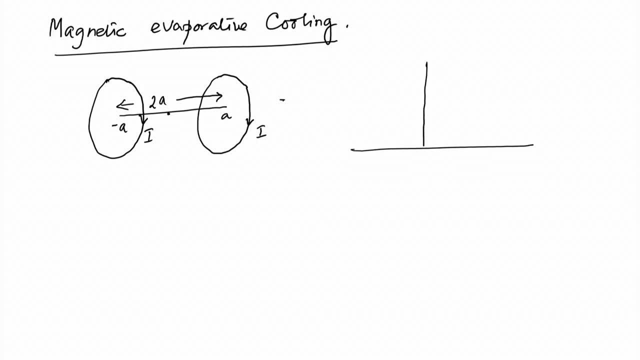 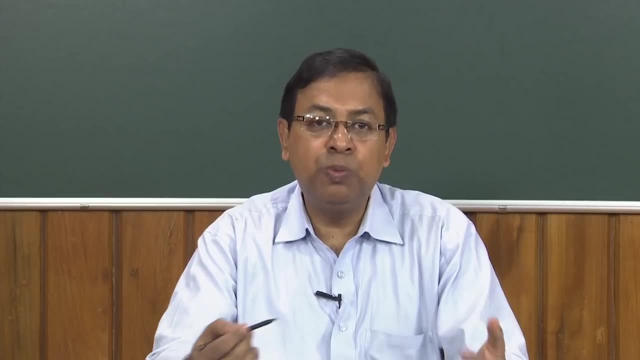 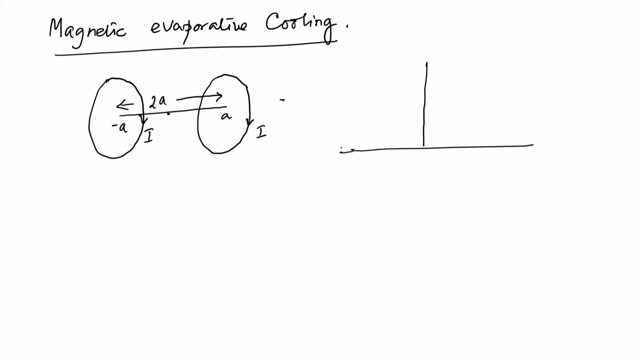 in the coil there will be generation of magnetic field Now, because there are two coils, so the magnetic field or the magnetic induction would be a superposition of the effect from both the coils and this would be like symmetrically it will. So these fall off as 1 over r, whereas it is fairly constant here, and this is a say. 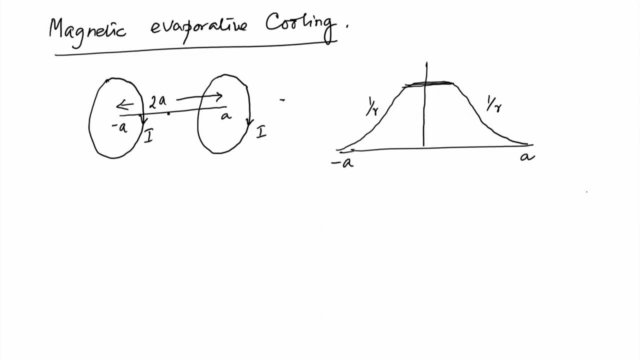 at minus a to plus a. So this is the situation for a Helmholtz coil, Or Helmholtz double coil, as it is said. Now, what person in MIT called David Pritchard did? he produced a similar coil with again 2 such coils. However, now the currents are: 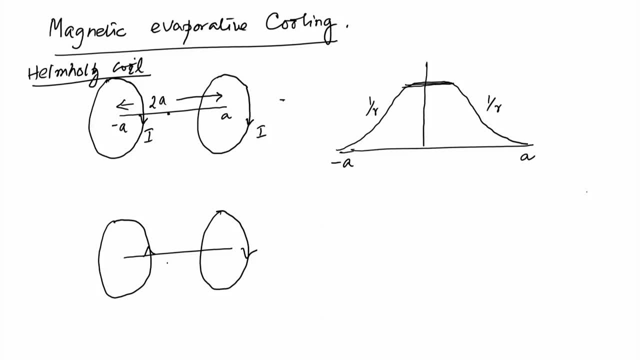 flowing in different directions in both the coils, so one with respect to the other, and now you will have a magnetic field variation, to be having a minima as opposed to a maxima, and which you can do a simple calculation to see. that is, it is, of course, symmetric. 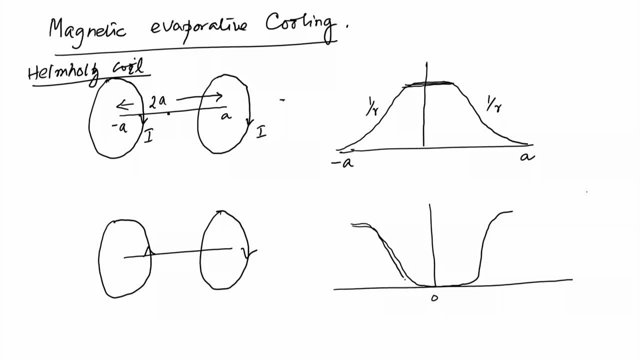 about 0.. Probably I did not draw it as symmetric, but it is beautiful. 3.101 has no change over. yes, this is, this is just 0, this is also zero. zero may not be terrific value and it is crisp. you will feel what when. k is 0, power minus 2 into at m bar. if I say can G at k using it, then it is no positive value. Then the unfficients coming after it becomes an inverse of x, P, x, 1 x 3, so either is something, else, only one is burnt out. 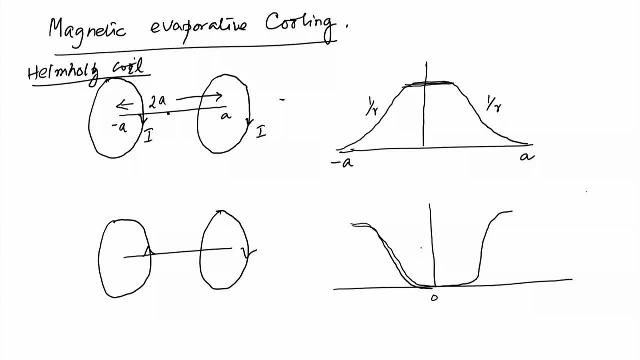 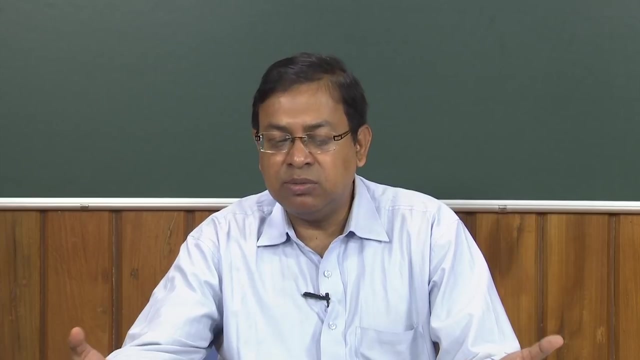 So this: if you can load the atoms here, then this acts like a trap for it. it is a magnetic trap for it. So any atom which has more energy will actually escape. So atoms will escape and leaving only say something like 10 to the power, 9 number of atoms in the system. 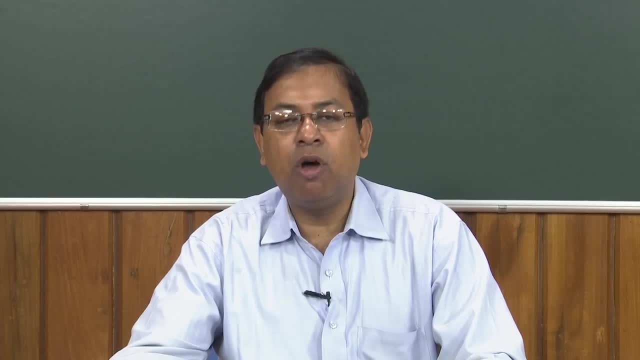 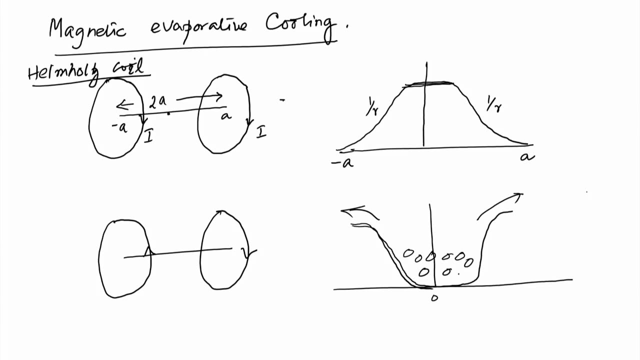 which is still, you know it is far away from BEC because BEC requires something around 10 to the power 6 number of atoms. But at least this does one step and it makes a lot of atoms which have which are energetically more, I mean they have higher energy, the energetically 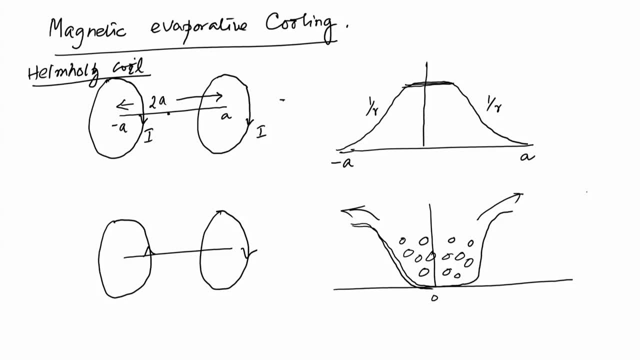 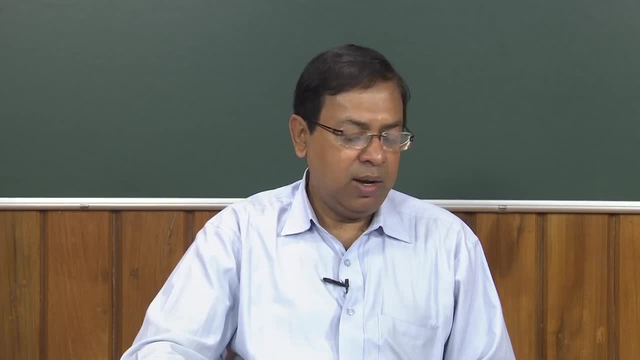 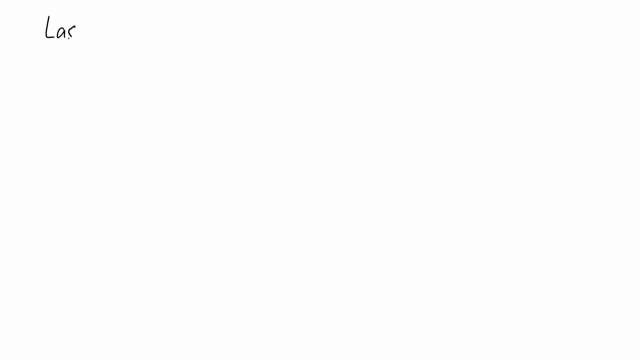 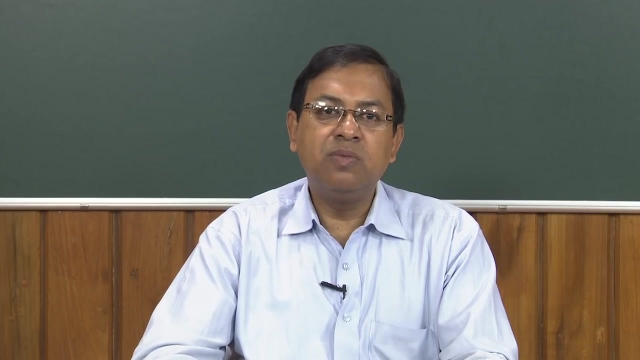 more favourable atoms would escape and leaving behind the slower ones. So we have a gas of cool atoms. So this is a one technique. the other one, as we said, that the laser cooling. So this is a very nice technique to slow down atoms and hence strip their kinetic energies and 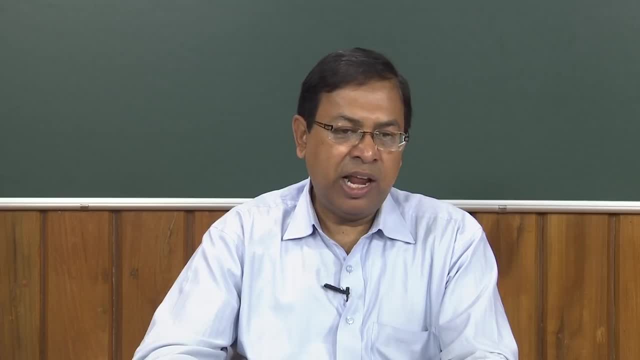 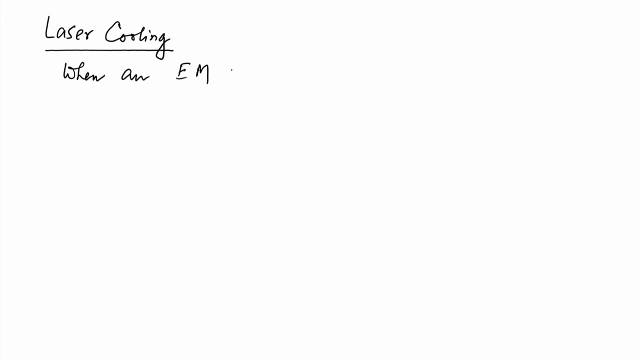 thereby reducing the temperature. Now notice that when an electromagnetic radiation of frequency omega falls on an atom- McDonough Нам Atom- whose energy level are given by omega naught or h cross omega naught, then this I will do without proof. 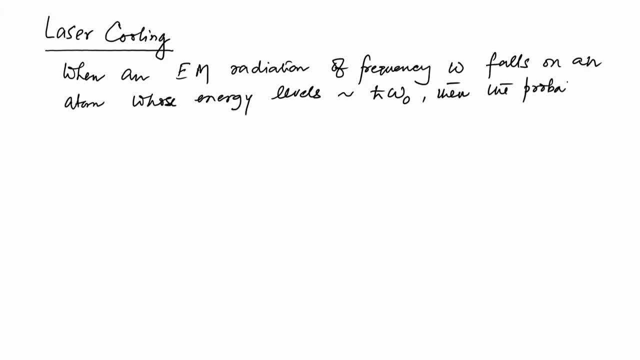 then the probability amplitude for absorption is proportional to 1 divided by omega minus omega naught, plus some I gamma, by 2, where gamma is the line width. It is the line width of the radiation, it is a natural line width. So this happens when the atom is at rest. but when the atom is moving, then the Doppler 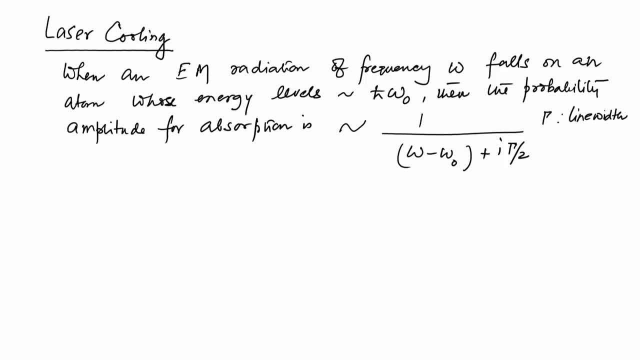 effect comes into play and if let me write this, 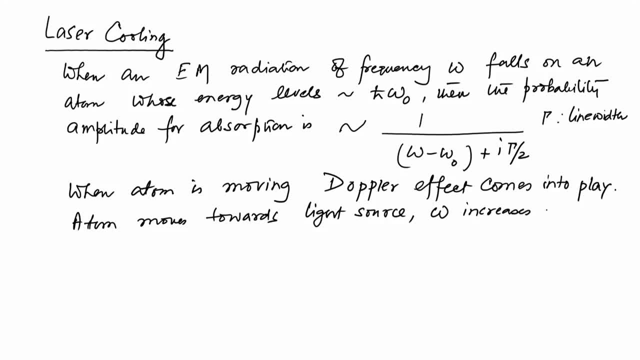 increases, the effective omega increases, and this is called as blue shift. And when the reverse happens, that is, atoms moves away from light source, omega decreases, and this is called as red shift. So this shift in frequency is, say, equal to delta omega, which is of, has a form which is v dot k with, or a minus, say v dot k where 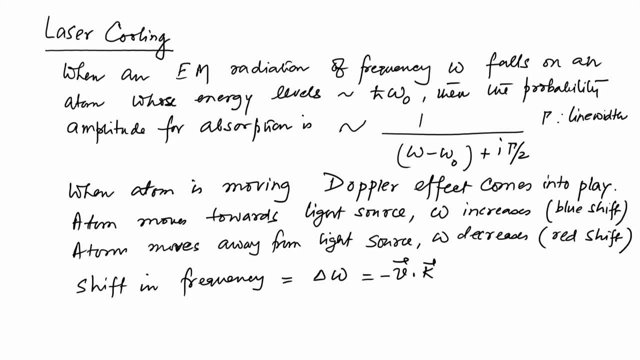 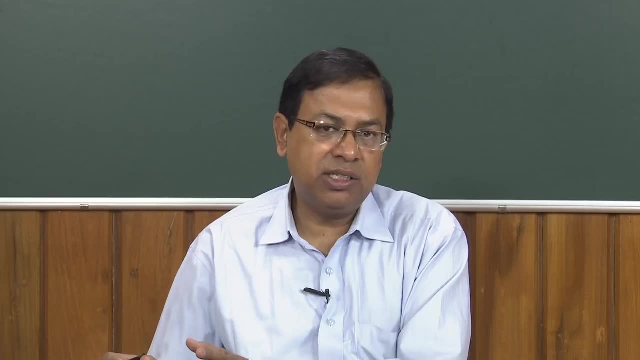 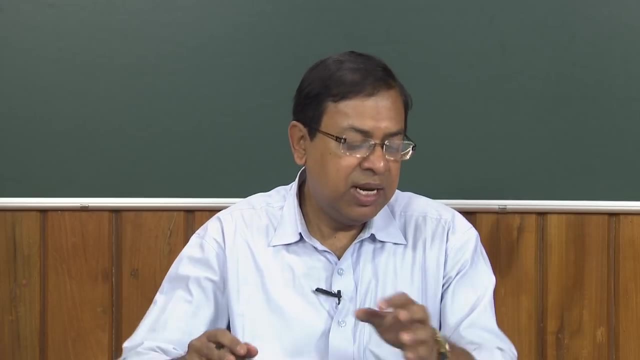 v is the velocity of the atom And k is the momentum. So if you need to slow down atoms then it is beneficial for the atoms to be moving towards the light source or the incident radiation. So if you can make the atoms move towards the light source then they will slow down and slowing down. 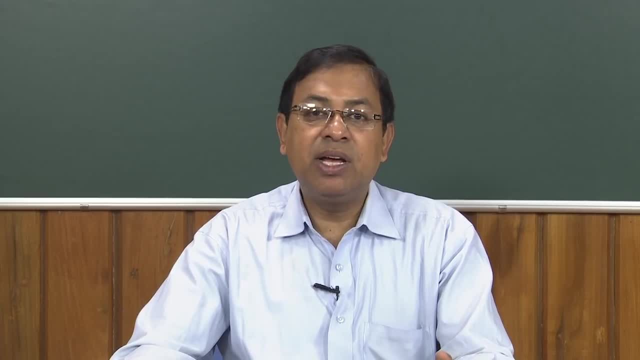 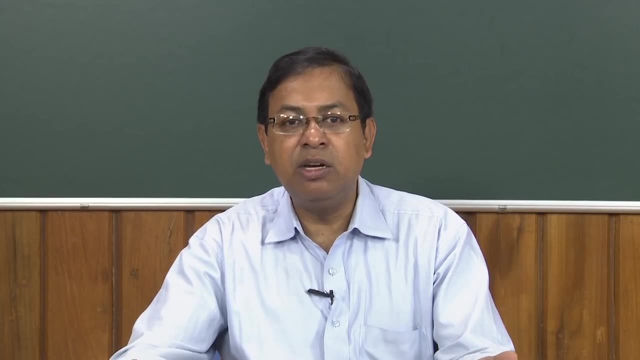 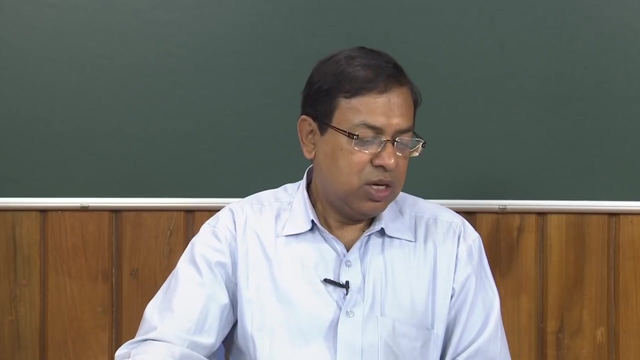 means the kinetic energy becomes less. and when the kinetic energy becomes less, the equivalent temperature, because the energy is always expressible in terms of temperature, with the Boltzmann relation E equal to k T, So the T decreases. So what happens is that the 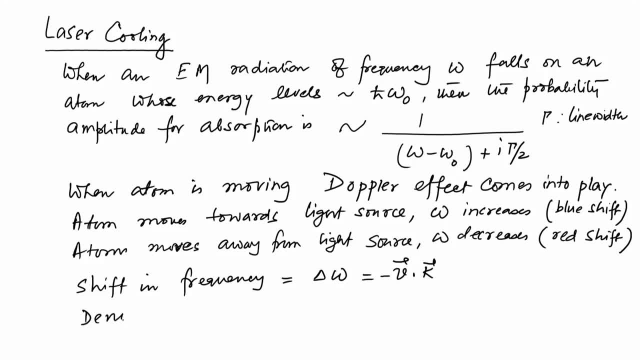 denominator here. So this denominator, it takes a form of omega minus omega naught minus v dot k. So this is a form of omega minus omega naught minus v dot k. So this is a form of omega minus omega naught minus v dot k. So this is a form of omega minus omega. 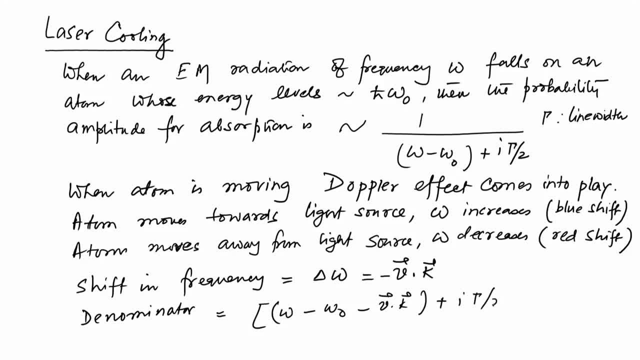 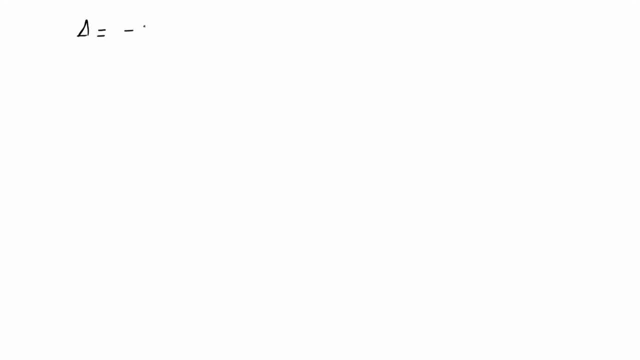 naught minus v dot k plus i gamma by 2, and so the quantity, So delta, is equal to minus omega plus omega 0, or rather omega naught minus omega 0 is called as the detuning parameter. So the dot k is equal to k T plus i gamma. 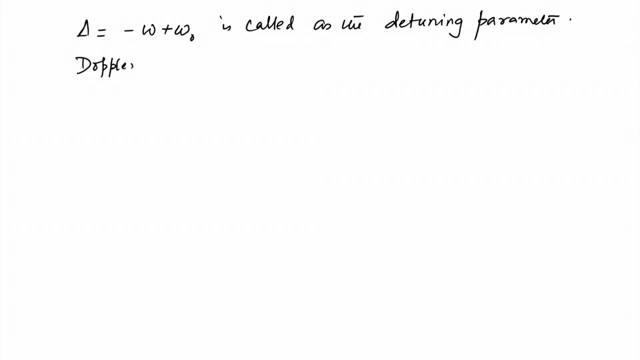 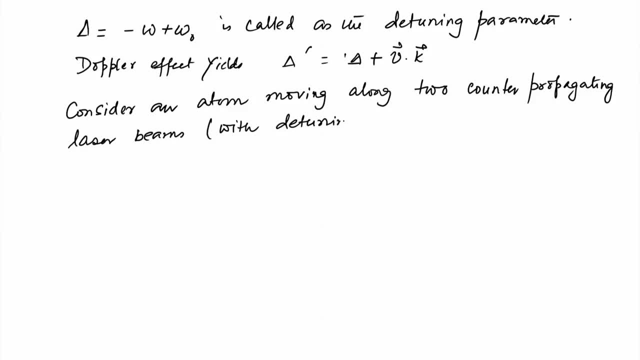 Then for both of them, for both delta 1 prime, that is this one, is equal to delta V k. So this is a 0 angle between them. So it is a V k cos theta, but cos theta is equal. 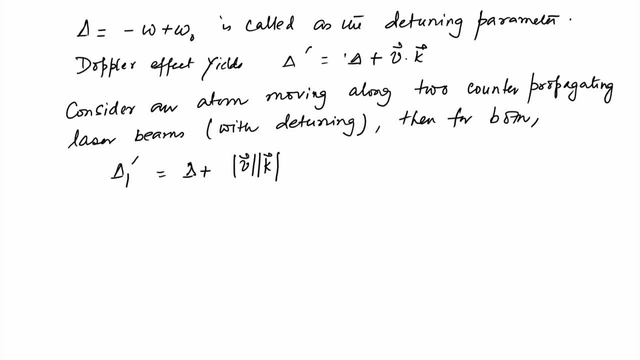 to 0 because they are moving towards each other and the atom is moving along the line, So there is no angle that it is making. and delta 2 prime for the other beam it is equal to delta minus V k. So it is clear that the so more energy is actually absorbed from. 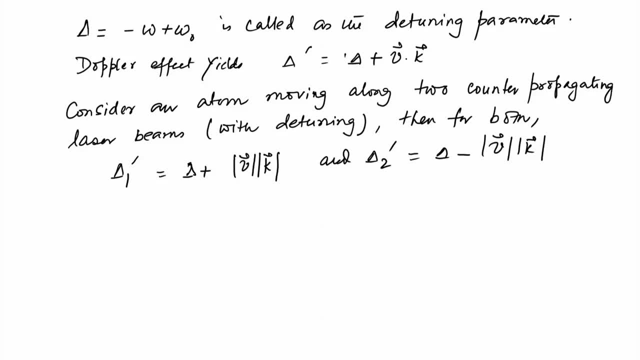 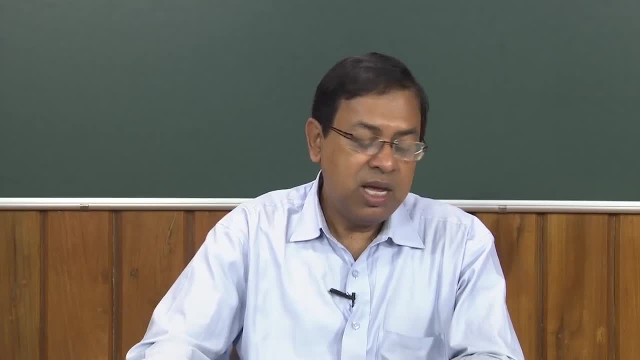 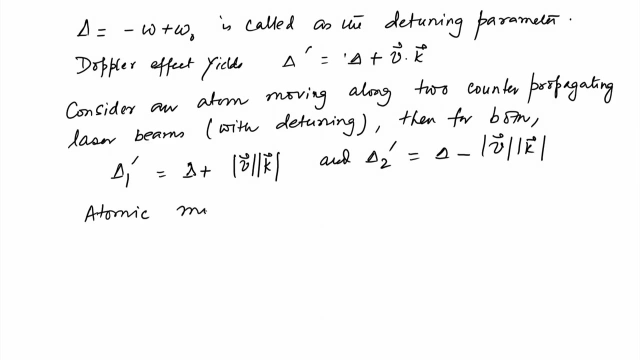 one of the beams as corresponding to the other. So we are talking about the two laser beams. So one of them is absorbing more energy from the atom as compared to the other. but this further means that the atomic momentum, The kinetic energy, is reduced by twice of this k V divided by c. So this forces exerted. 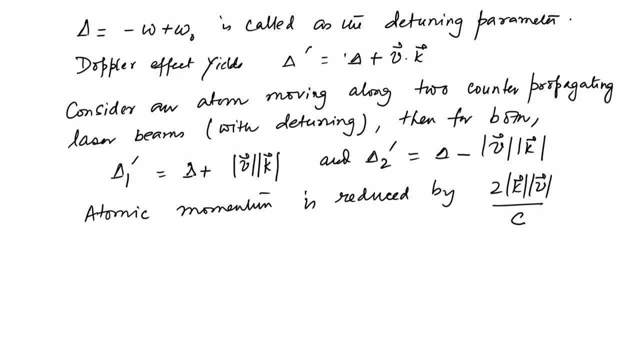 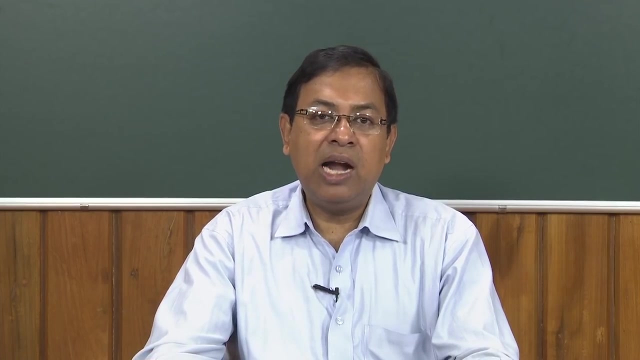 by the beams on the atoms are not balanced, So there is a resulting in a net force opposite to V and thereby reducing the kinetic energy And so reduces kinetic energy and causing cooling. Now this ends the story on cooling from our side. but you understand that all these engineering of having cold atoms possible, in 70 years and they are the best minds that were working in the subject. it still took a very long time for getting them down to a temperature which is extremely small and BEC really happens in sort of micro Kelvin in the micro Kelvin range. 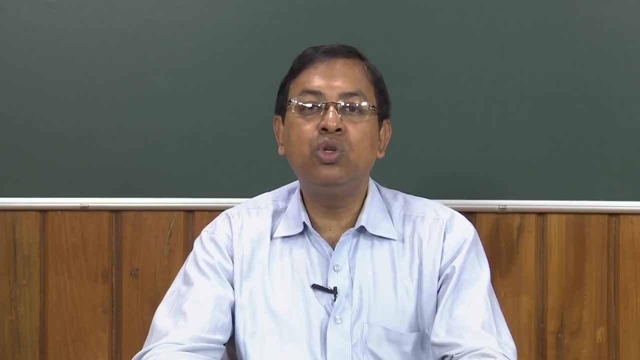 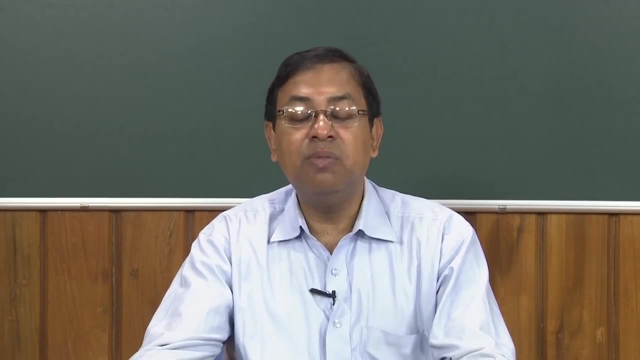 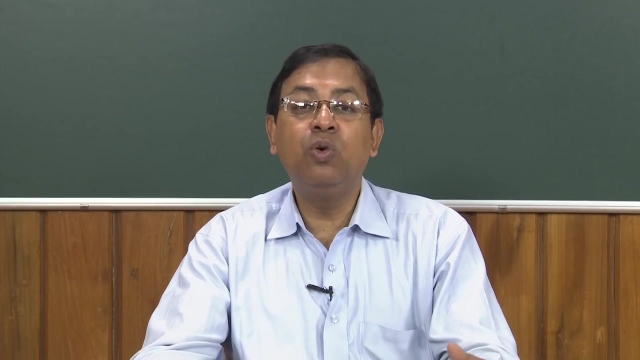 However, we will do a calculation and we will show that actually for the atoms such as helium, the condensation, or rather the condensation like temperature, is just about a few Kelvin, may be 2 to 3 Kelvin. However, understand that actually the rubidium atoms required. 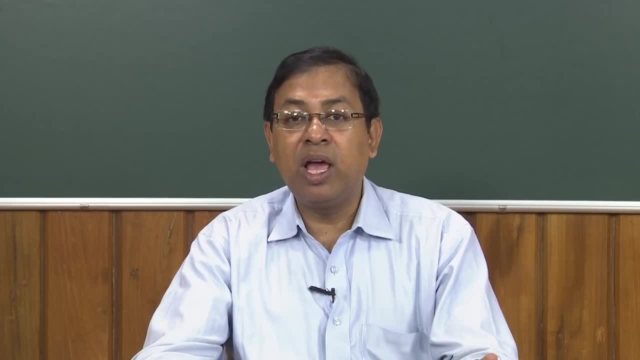 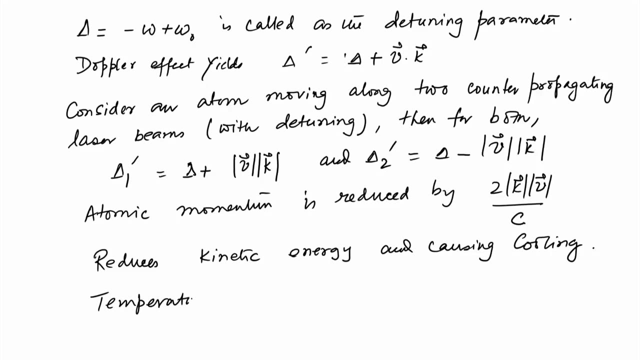 a temperature to be of the order of micro Kelvin and the. So let me write that the temperature is of the order of. finally, and this is only a part of the cooling techniques that I have talked about, There are the Sisyphus carbonate, the, in several 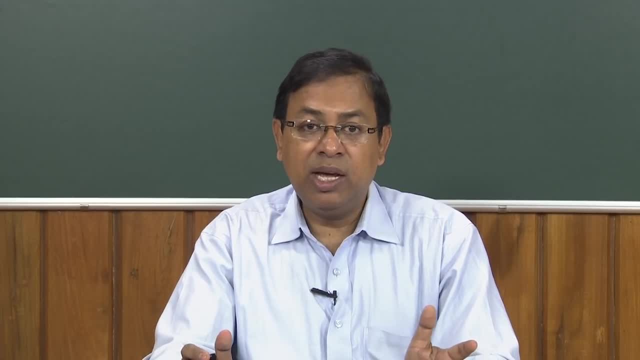 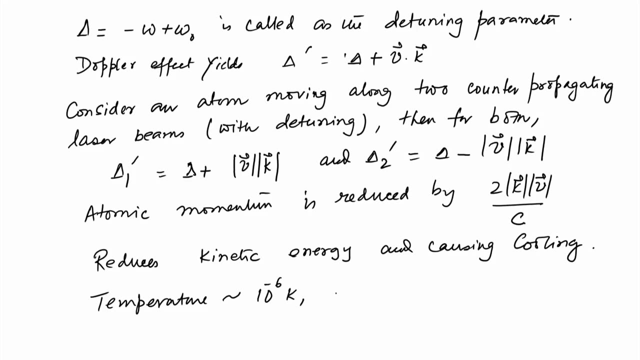 cooling and sympathetic cooling and so on, And so this temperature comes to about 10 to the power minus 6 Kelvin, and the number of atoms or number of particles that should be left is about 10 to the power 6.. So this is the condition for BEC to be. 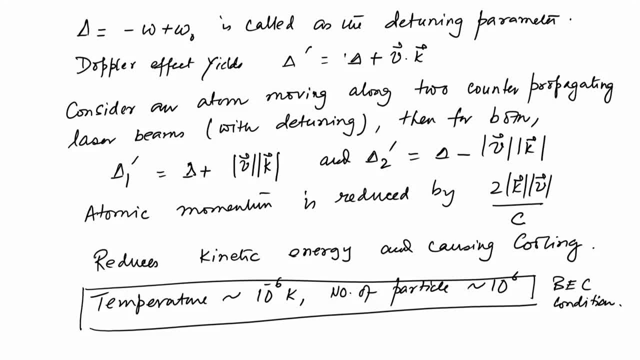 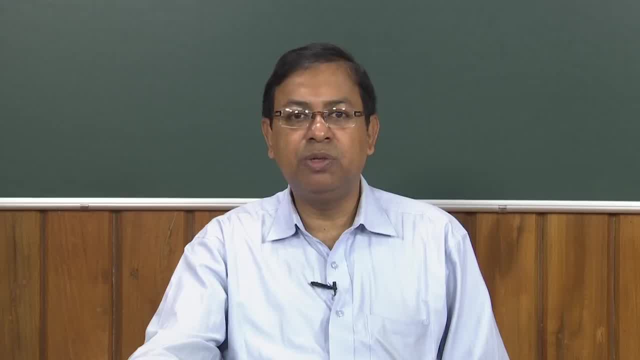 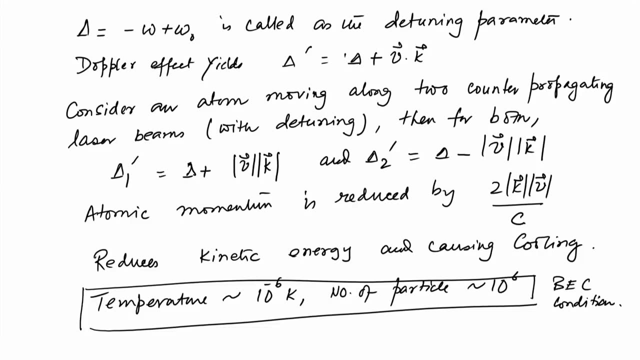 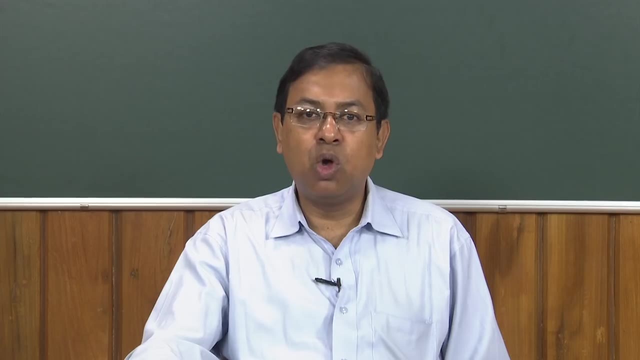 formed in lab and however, as I said, that will not, will not discuss the exact magnitude of the temperature, but will do an order of magnitude calculation. Now, since we are done with the cooling part, let us understand that. why is that we are talking about a bosonic atoms, when the atoms are actually neutral, or rather the charge? 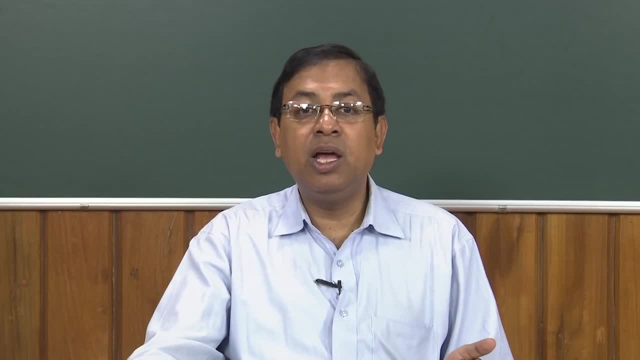 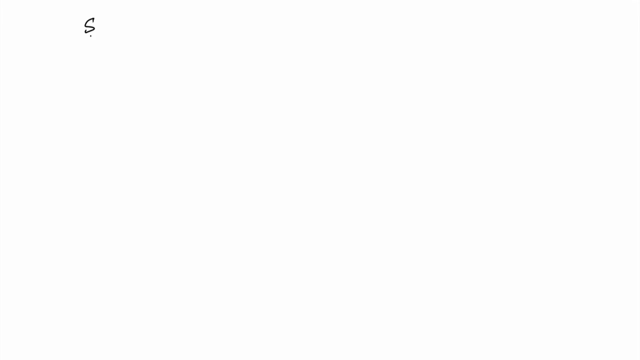 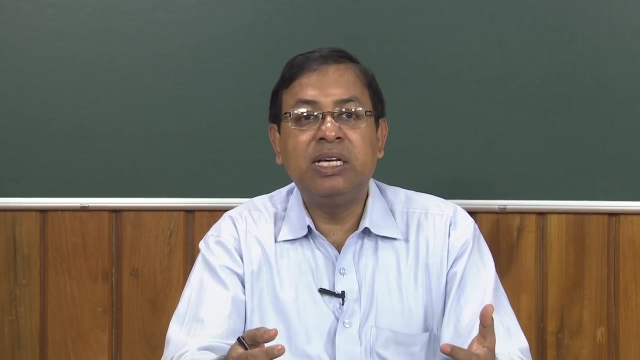 neutral. And if we are talking about the electronic, the spin, then that electronic spin is always half and these alkali atoms, rubidium being an alkali atom, So this that should correspond to electrons having a spin half and that cannot be put in the same class as 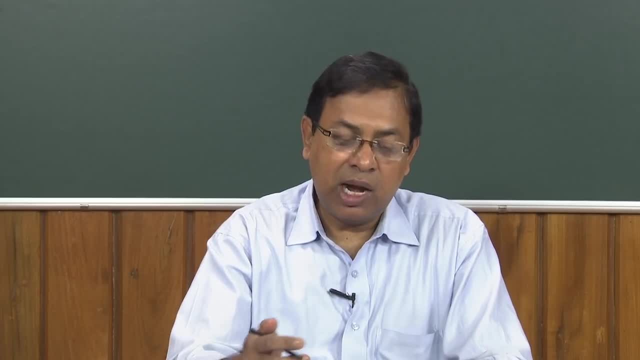 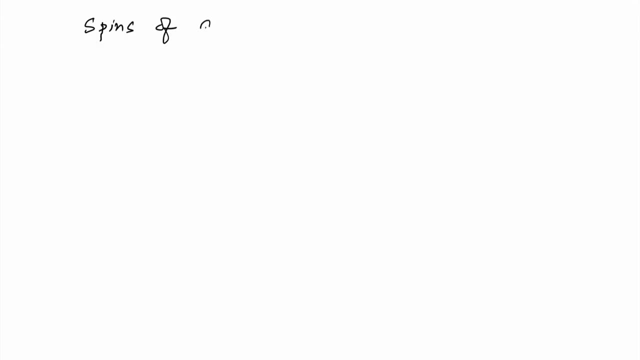 bosonic atom. So let us understand why they called as bosonic atoms. we are just talking about alkali atoms, because it started with alkali atoms, as I have shown you: rubidium, sodium, etcetera, potassium, lithium again. So what happens? 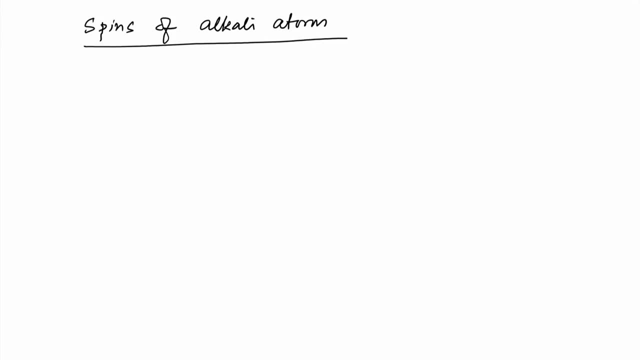 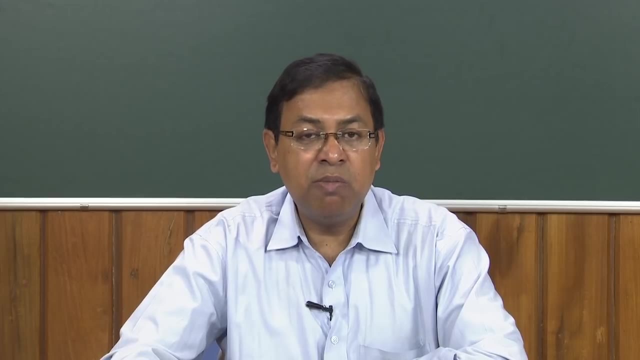 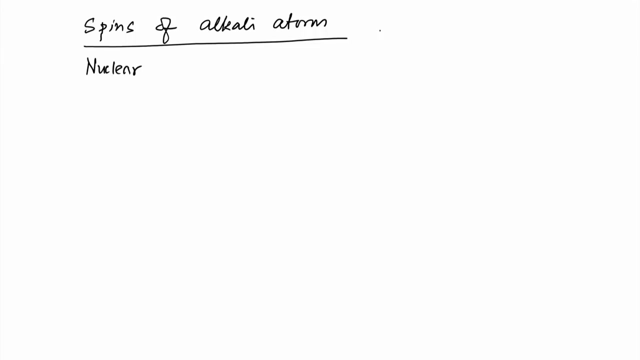 is that even if the electrons have the spin, half it is the nuclear spin. So it has the nuclear spin that comes into picture, but because the nuclear magnetic moment Mue n tear. 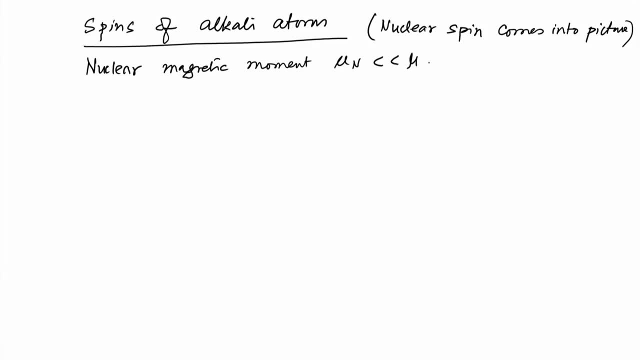 is far lower than mu E, which is a nuclear magnetic moment for electrons, by at least 4 orders of magnitude, And thus to have nuclear spins to play an important role, we really need very low temperature. So let us say that F is the atomic spin, I is the nuclear 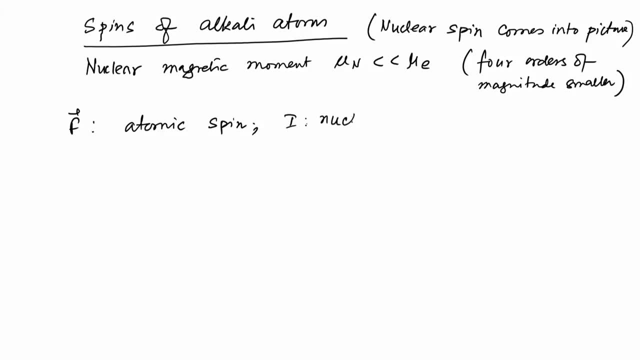 spin and J is the electronic spin. So F is equal to I plus J, and so it has a range I plus J to I minus J, and for J equal to which is the electronic spin equal to half. So we have F. and for rubidium: ok, let us. 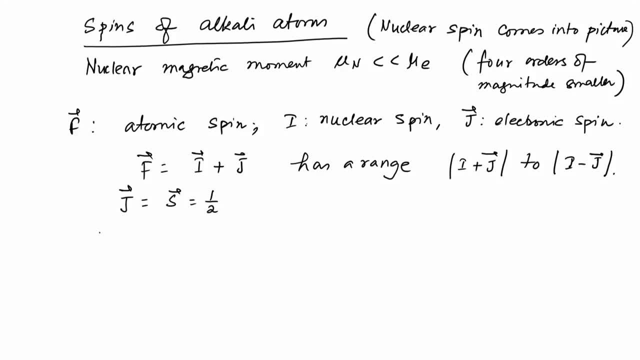 consider for the alkali atoms such as rubidium, sodium, lithium, etcetera, we have I, which is the nuclear spin, is 3 by 2.. 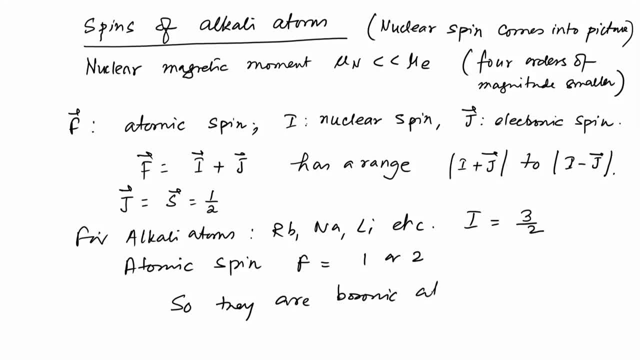 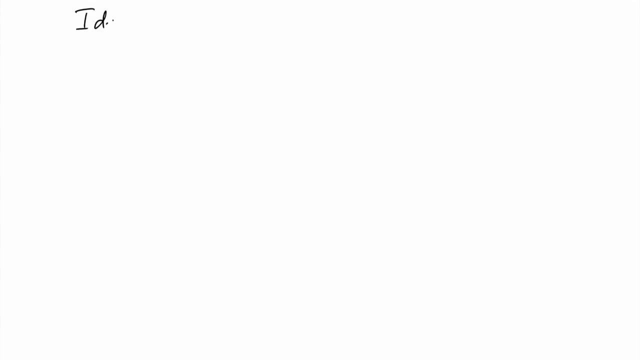 delimitation phenomena in a ideal Bose gas. so let us start with the ideal Bose gas and the discussion is: you can follow statistical. 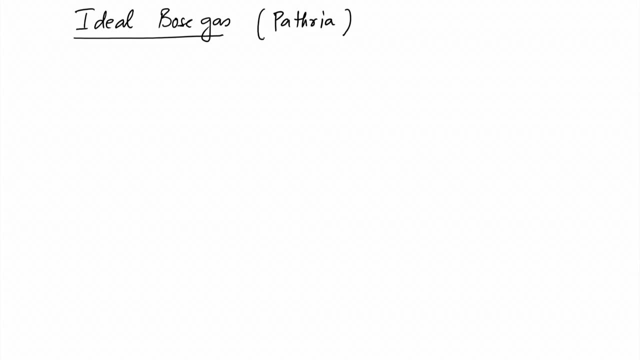 mechanics book, very good statistical mechanics book by Parthia which gives a very good description of this phenomenon. Before we 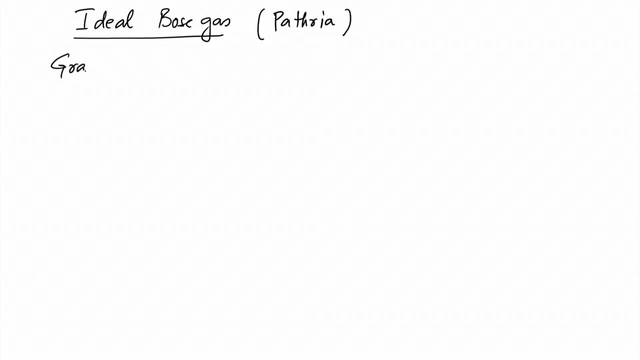 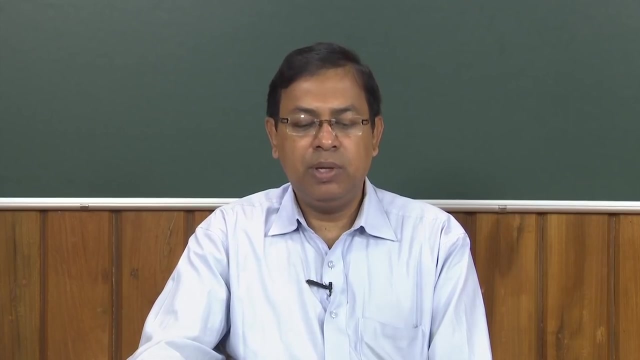 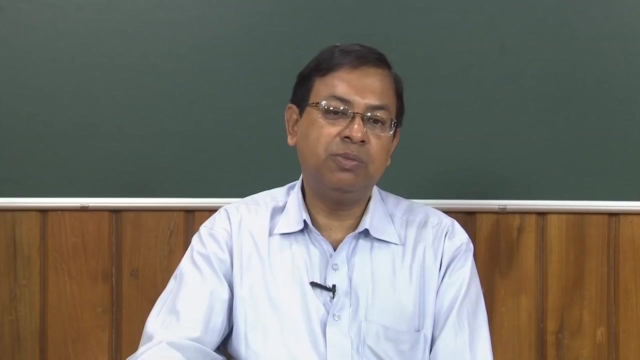 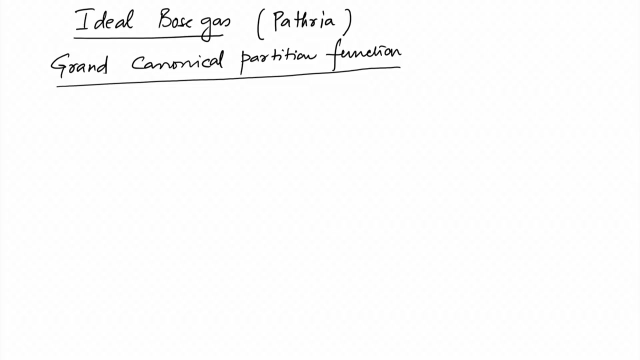 proceed. let us write down the grand canonical partition function. So the word grand canonical, grand canonical partition function is that where we also allow, in addition to exchange of energy among the particles, we also allow for exchange of particles between the system and the bath. So it is the canonical is about exchanging energies between the system and 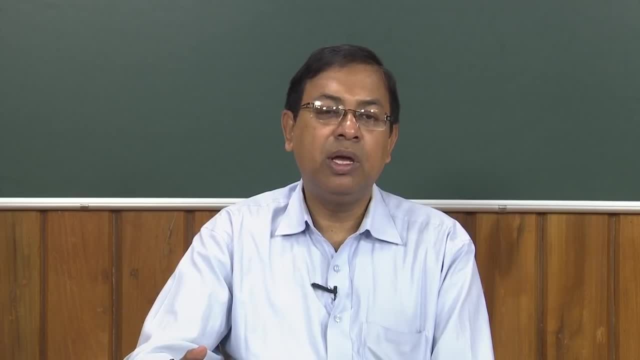 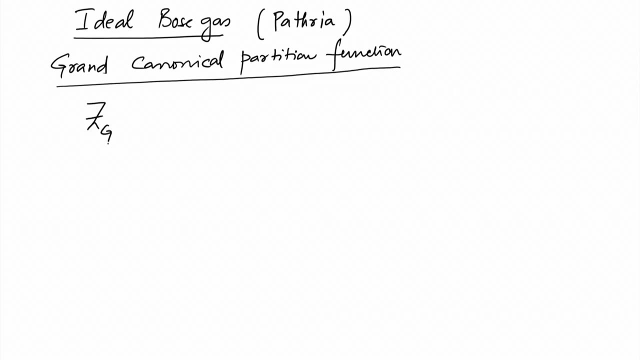 the bath. and this is also, in addition to that, allowing the number of particles. So the number of particles is not constant. So grand canonical partition function. as you know that the partition function is written with Z and this Z comes from German word, probably. 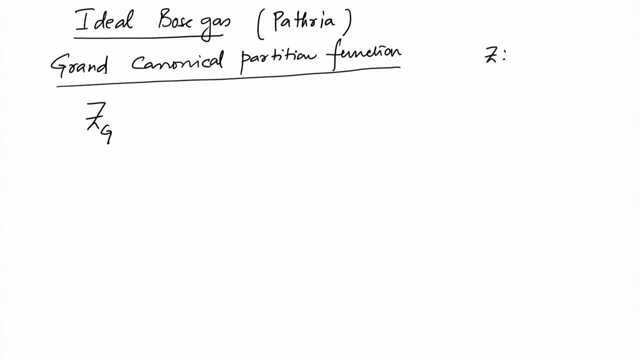 it is called, as there could be a problem with the spelling, but it means systems. who may, means that it is a sum over states. So G, subscript G, that corresponds to the grand canonical. So this is equal to n, equal to 0, to infinity. as we just said that we will allow the particles to be exchanged between: 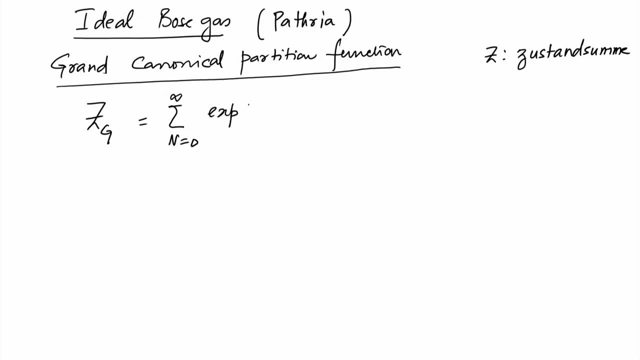 the system and the bath. So that is that term. and exponential beta mu n, and this is equal to an exponential minus beta. epsilon i, n, i and sum over others, over all states, let us, you know, you can write n, i and so on. So this is the canonical partition. 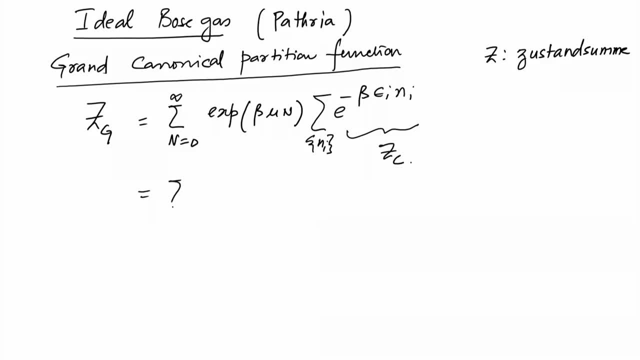 function, and so it is basically n equal to 0, to infinity exponential beta, mu, n, Z, c is pretty much the formula for the grand canonical partition function, And you can follow path here to see that the grand canonical partition function, the log of that which is related to the free energy, a minus K, T of that is equal to F, which is 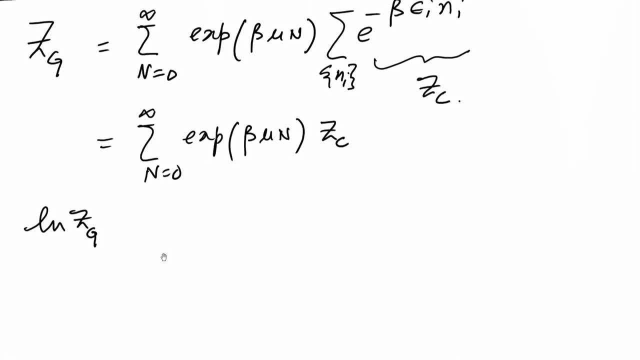 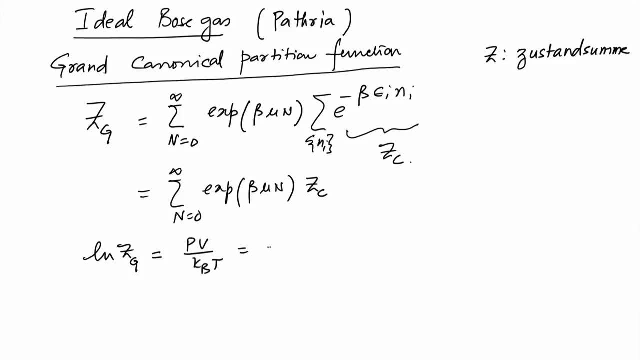 equal to P v. So this is equal to P v over K T and which is equal to a minus sum over i log of 1 minus Z f. I will write for t. So f is equal to theta epsilon i, and where z F and beta epsilon i and so on. So let 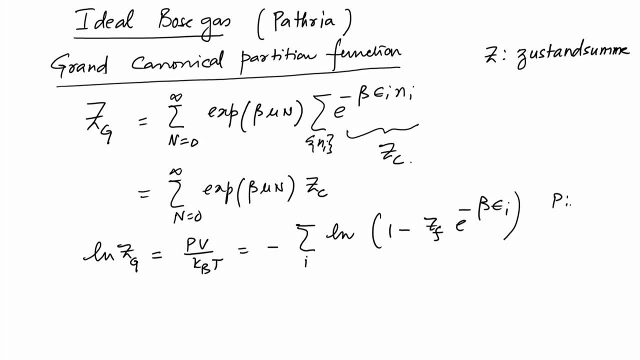 us make this notations all clear. So p is equal to pressure, v to be volume, t is of course temperature, Z, f is called as a fugacity, which is equal to exponential beta, nu, beta i is 1 over K T, the. So let us write it here: mu is chemical potential. 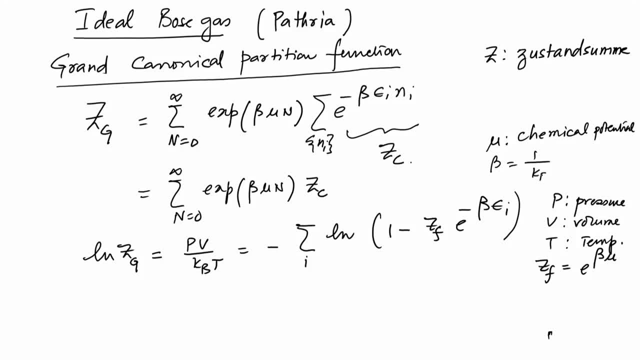 and beta equal to 1 over k T, and So this is by and large the expression for this. So this can actually be the equation of state for an ideal Bose gas, because we are writing P V by k T, which, you know, for a classical ideal gas, P V by k T is equal to some R or 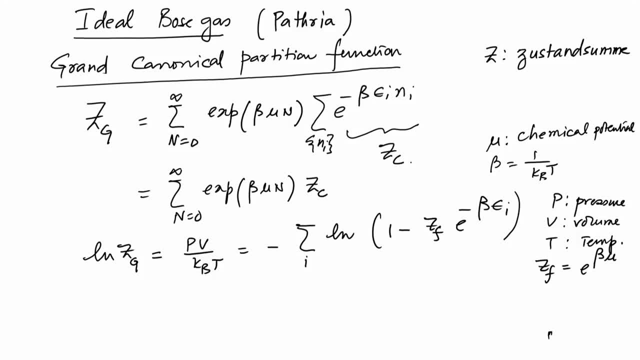 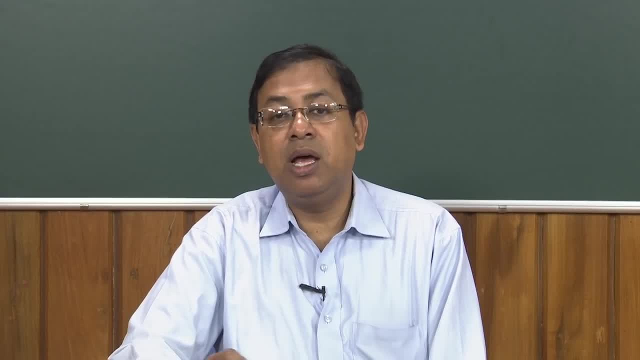 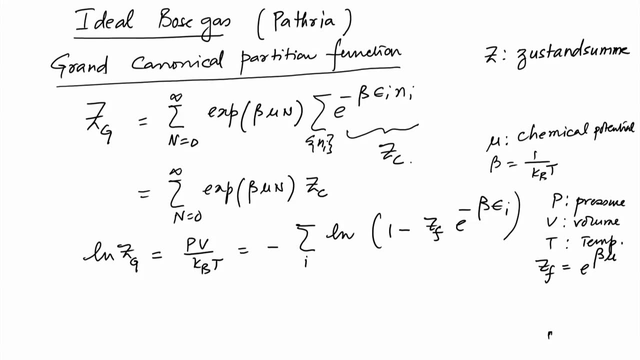 it is N, R or something like that, So it is a constant, whereas in an ideal Bose gas, a quantum gas which follows, an indistinguishability constraint is given by this And similarly the number of particle, which is equal to sum over I. 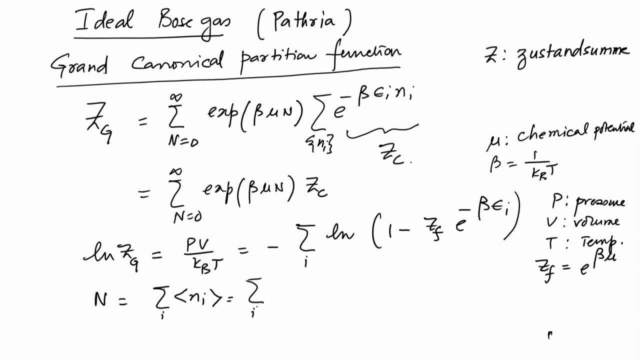 So N I. this is equal to sum over I and 1 divided by Z F inverse, or you can simply write it as: exponential minus beta mu and exponential minus beta epsilon I plus this is minus 1. sorry, So for boson is minus 1 and for fermions it is equal to plus 1.. Epsilon I s are the. 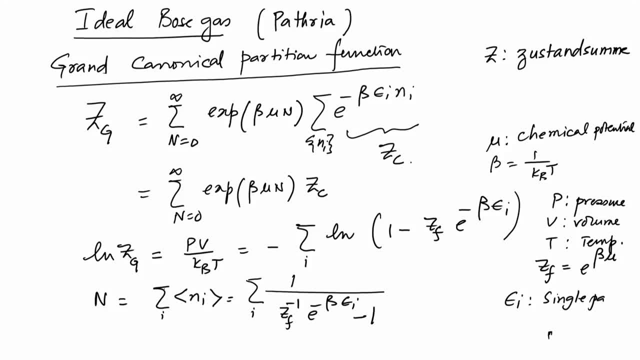 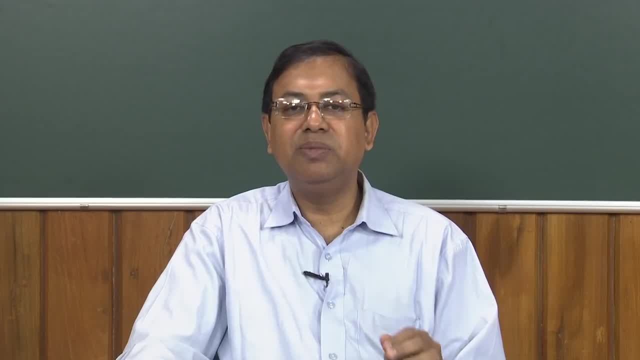 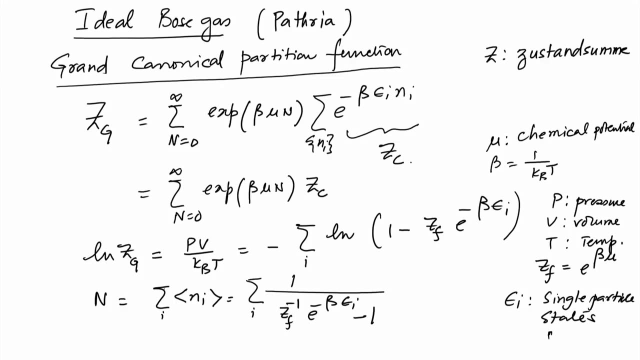 single particle states. So what I mean by single particle states is that if they are free particles, so they will go as the in case phase, they will go as h cross square, k square over 2M. Now, before we proceed, what we have to do is that we have to convert these, or rather, 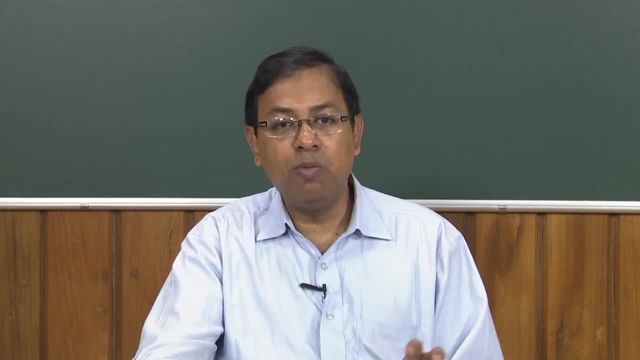 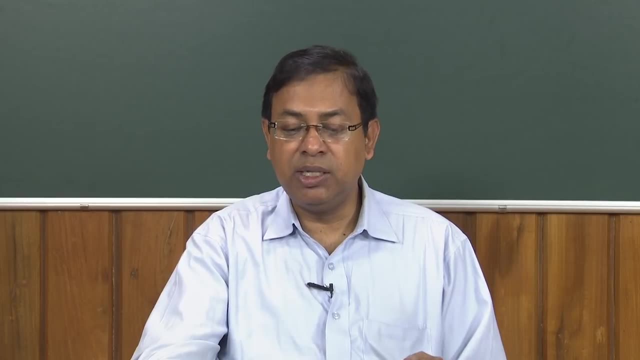 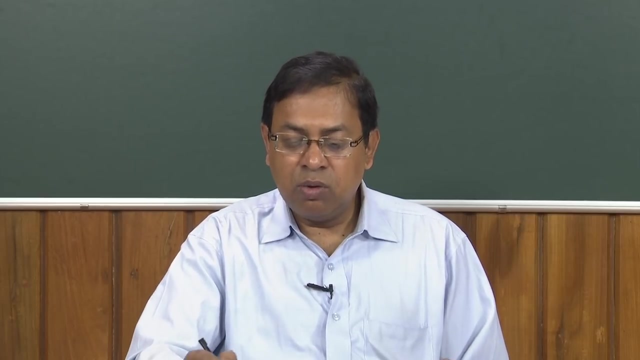 these are the working equations for any system, whether you are talking about condensation or you are talking about studying other thermodynamic or statistical mechanics and mechanical properties. mechanical properties: you have to start with these equations for both fermions and bosons. Now we need, in order to calculate them, we need to calculate them analytically, we need: 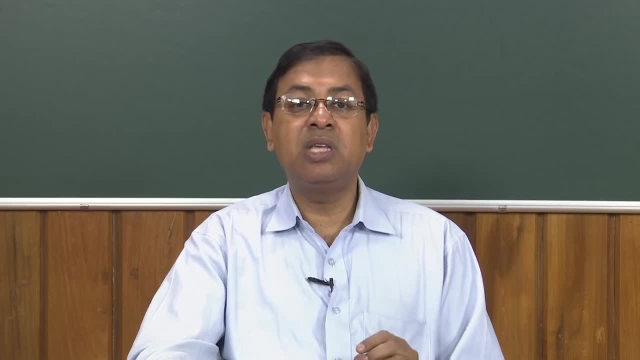 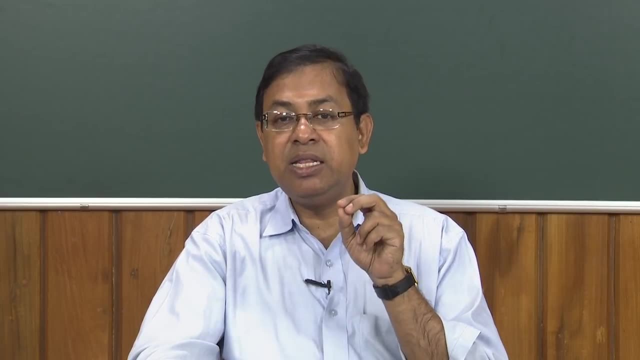 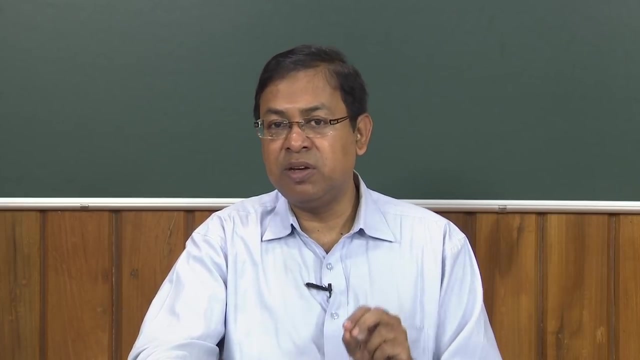 to convert them into integrals. And you know when a sum is converted to an integral. you need the density of states, you need the number of states in the energy range E and E plus dE, And that is an important quantity in condensed matter physics, as I might have already told. 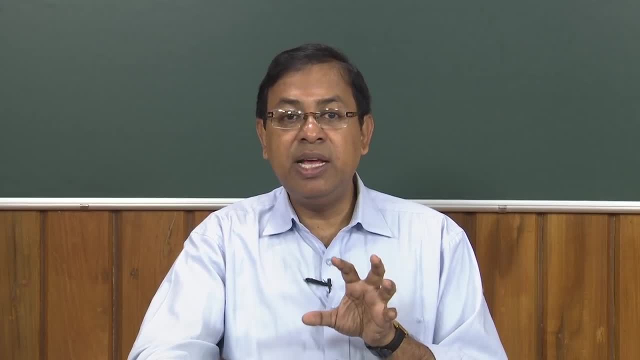 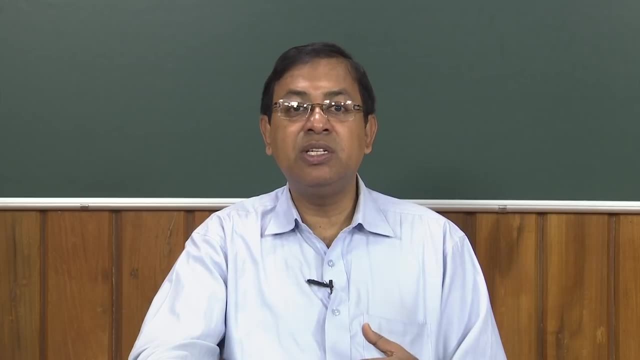 a number of times, because this is what creates a difference between a two dimensional, the properties of a two dimensional system, with that of a three dimension, because the density of states goes down. In fact, the nano, the whole branch of nanoscience and nanotechnology- 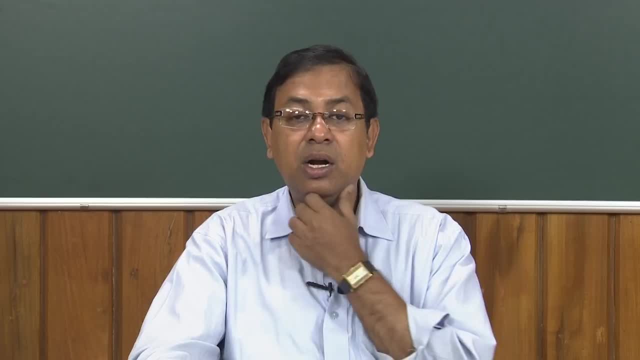 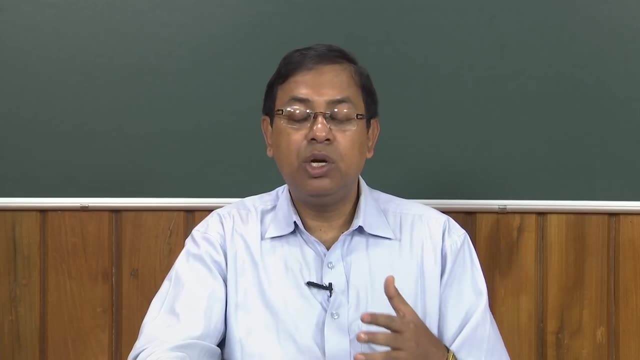 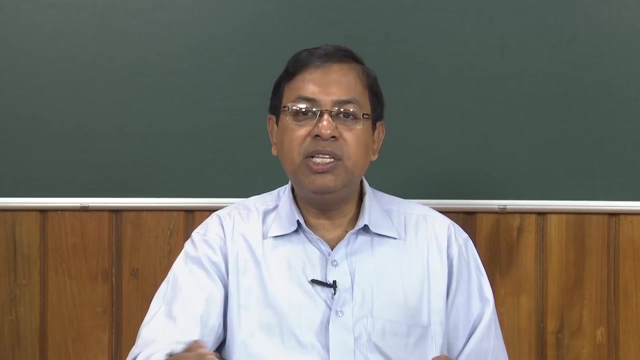 when we talk about quantum wires, which means that we are confining electrons of the charge carrier in one dimension, While in quantum dots we do it in zero dimension and in a two dimensional electron gas this is in two dimension, and so on. So we need the density of states in order to calculate. 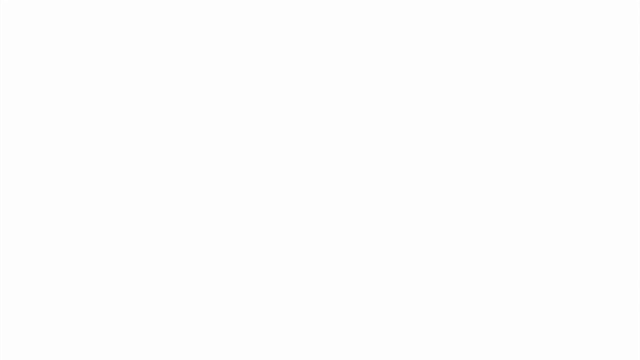 or rather convert the sums into integrals. Now this is, I will not go into that, but it is a very simple calculation. first course of solid state physics would do it that the density of states, in short called as a DOS. So that goes as epsilon to the power, half for epsilon equal to h cross square, k square. 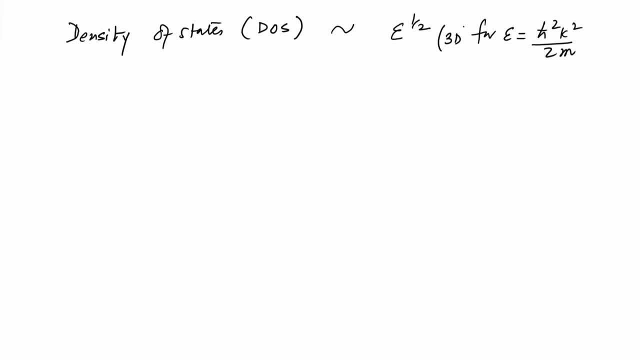 over 2 m. This is in 3 D. it goes as constant. also let us write it as epsilon- to the power 0, which is also which is a constant in 2 D, and it goes as epsilon to the power 0. So 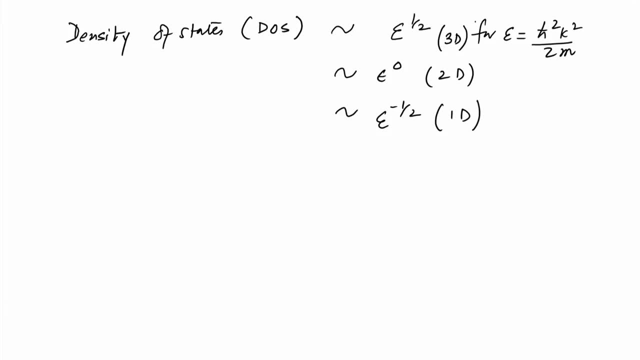 that goes as epsilon to the power minus half in 1 D. ok, So for this dispersion, a free particle dispersion. So if you see this, that the density of say. so we are talking about a three dimensional system with k square dispersion. So we are talking about a D dimensional system. 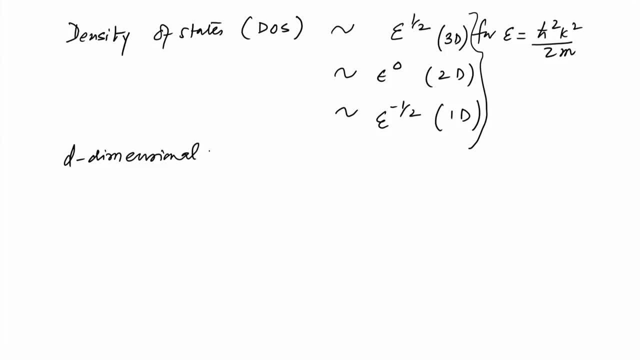 where D equal to 3.. So D equal to 3 for us, And we have a dispersion which is S going as So, dispersion going as k to the power S. So S is equal to, So S is equal to 2 for us. In fact, whether a BEC will occur or not will crucially depend. 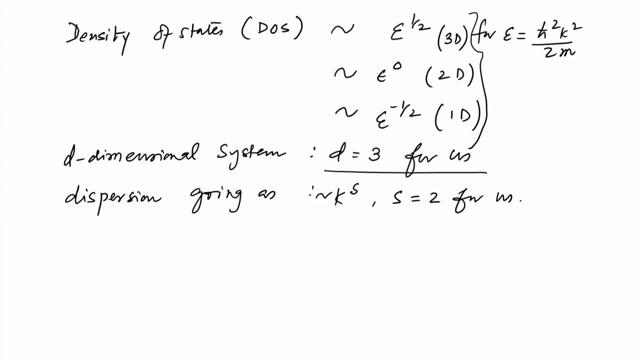 upon this value- D and S- and you can actually convert it into a single parameter. So either you call it S by D or D by S, So you can convert it into some certain values of S by D or D by S. it is Bose, Einstein condensation. 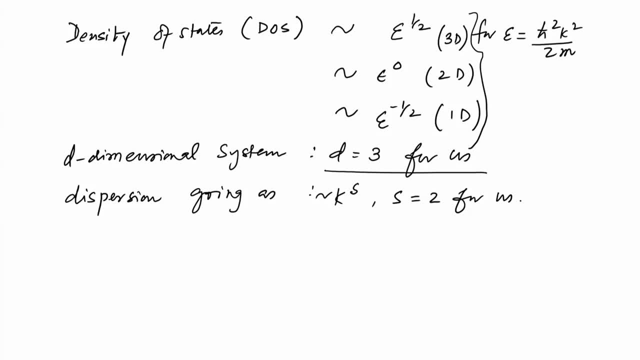 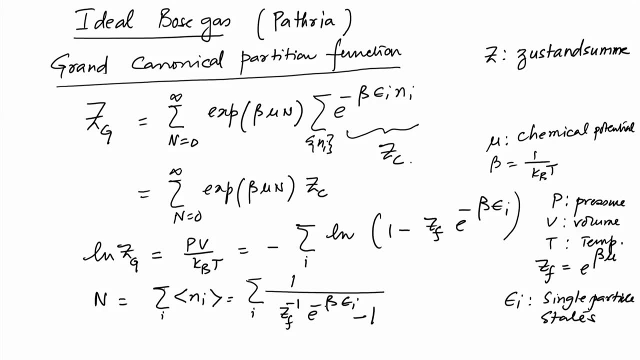 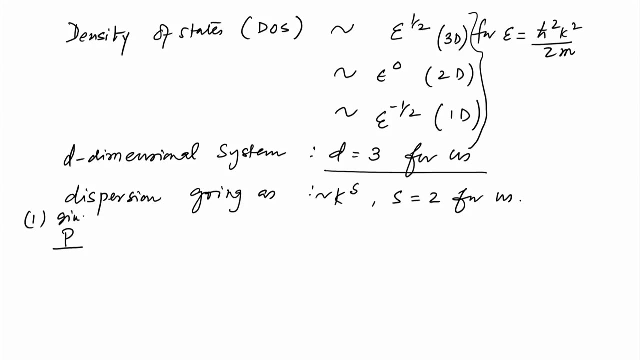 is possible. So we convert using this density of states. we convert the first equation- let us call them as a first equation- and second equation, and let us write: 1 gives, So 1 means equation 1 and. 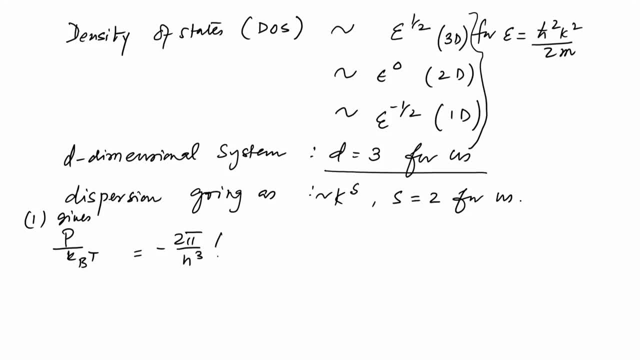 I should have actually done it for to all epsilon. 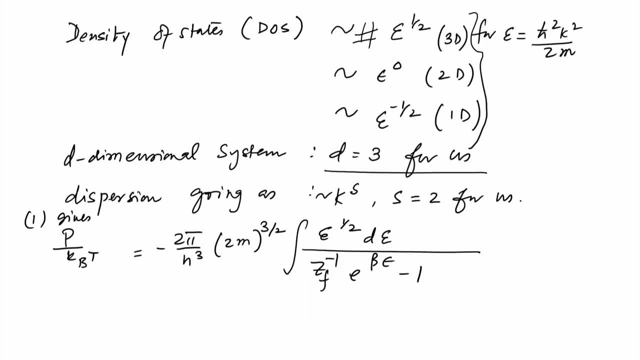 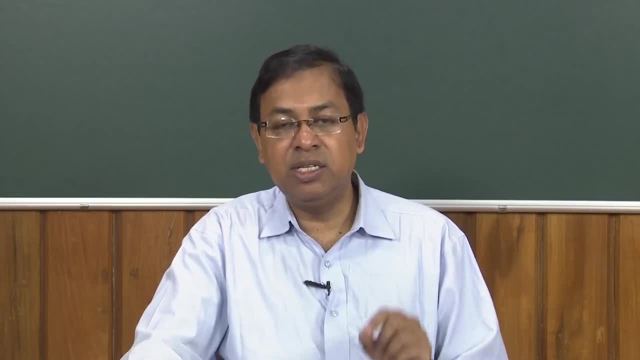 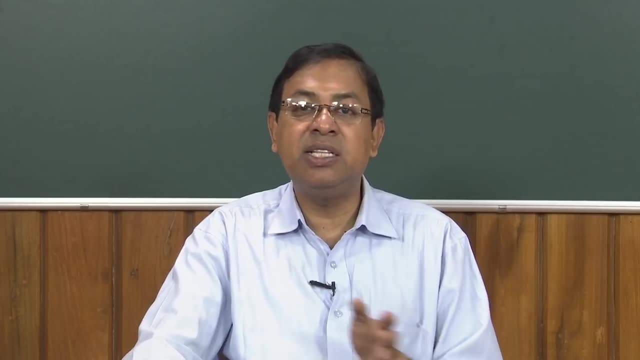 But, however you see, if we have epsilon to the power half and for the ground state, which is epsilon equal to 0, you would attach 0 weight. This what I was talking about earlier, that not have a 0 weight assigned to a given state, then that state is completely unimportant. 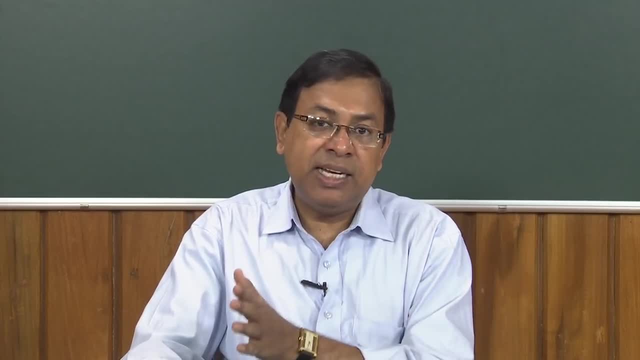 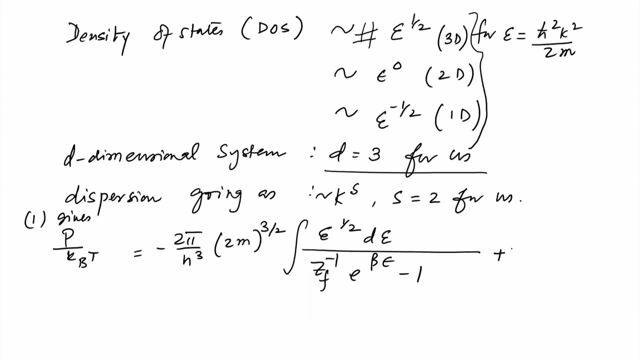 for our computation. So we will have to take that state out and write it for that state. we will write this thing as rather it is a minus sign, it is a minus 1 by V log of 1 minus Zf. So this is that contribution for the epsilon equal to 0, and this is for epsilon. 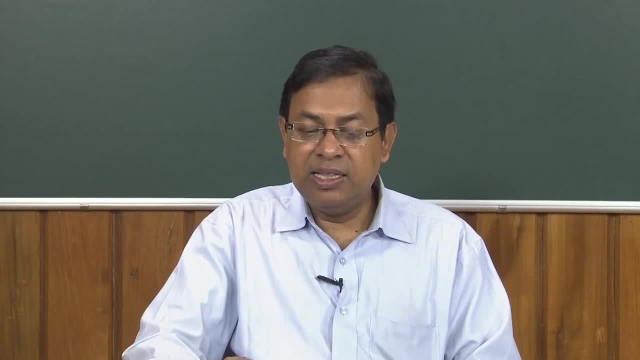 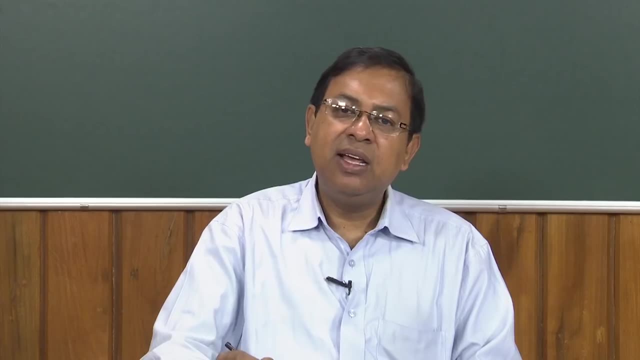 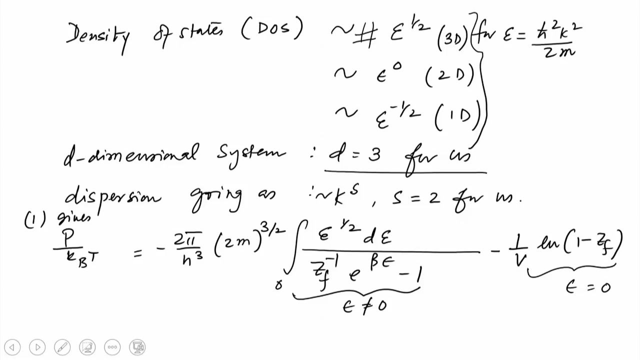 not equal to 0.. Now, ideally I in this integral we should separate out the epsilon equal to 0, but since this is an integral, just having one point less does not make any difference in this integral, So we can still put it as 0 to infinity. 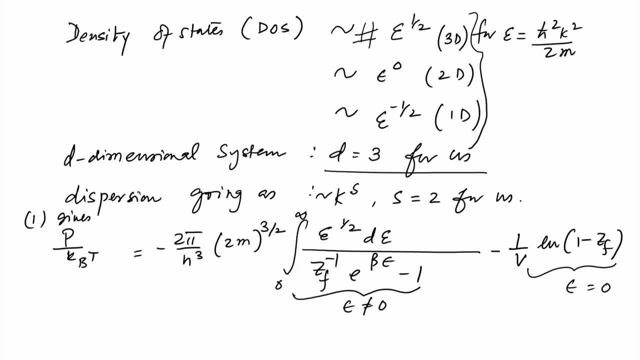 So so the integral, So integral, becomes 0 to infinity. and this integral, and then this is the epsilon, equal to 0, component of that equation, equation number 1.. So now let us call this as equation number 3 and 2 gives in the same manner: n by V is equal to 2 pi over H cube, 2 m by 3. 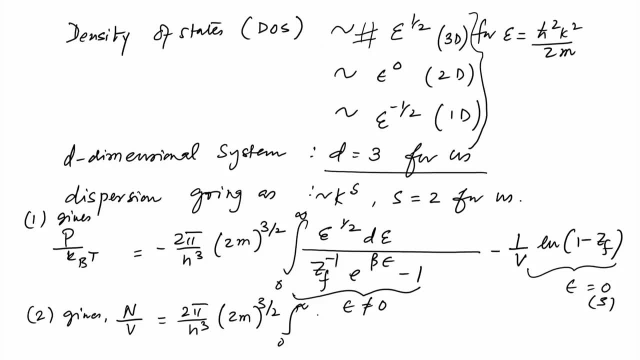 by 2. And 0 to infinity, just in the same way. and d epsilon, and you have a Z F inverse exponential beta epsilon minus 1 and the plus 1 over V Z F by 1 minus Z F. let us call this as equation. 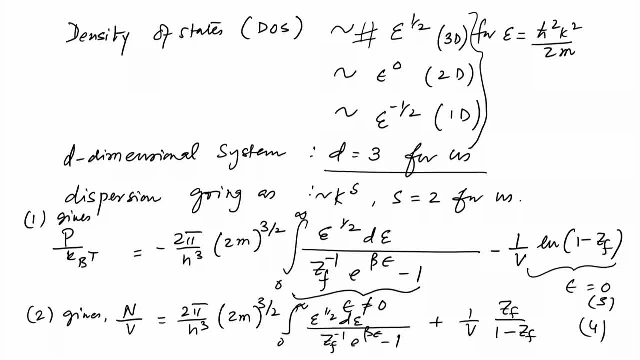 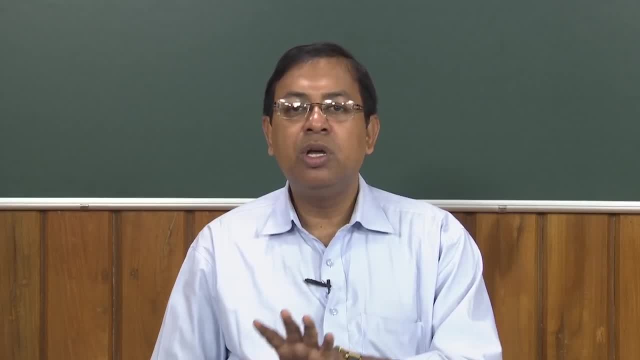 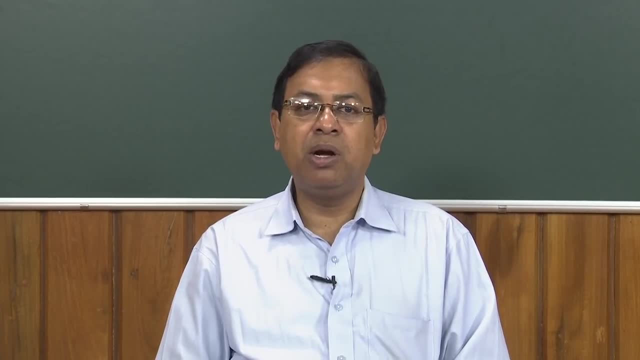 4.. Now, if you look at these two equations, we have clearly a separated them into two terms: one corresponding to epsilon equal to 0, the contribution to the pressure, corresponding to epsilon equal to 0, and the contribution to the density of particles, or the number of particles to be for epsilon equal to 0. 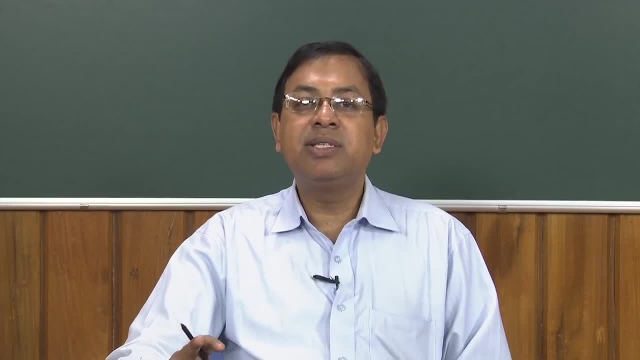 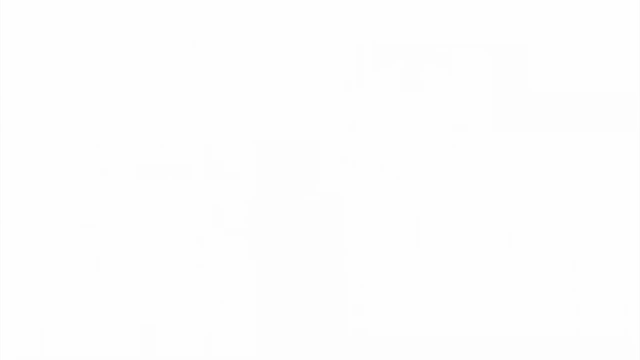 and for epsilon not equal to 0.. This is in one of my slides that I have shown the ground state energy to be separate as compared to the excited state energies. So now let us see the second terms of both, the of both 3 and 4.. So, see what the second terms are, let us write that second term as: 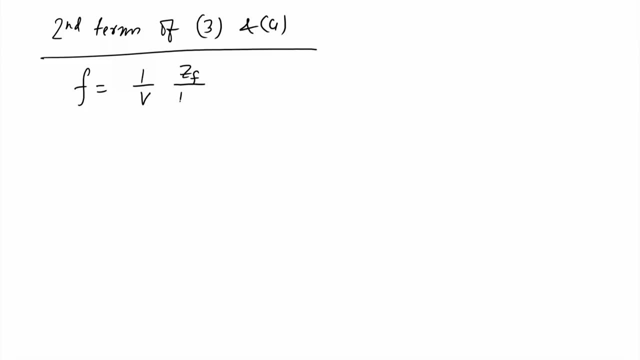 this. it is equal to Z F, 1 minus Z F, and that is equal to N naught by V. you understand N naught. N naught is the occupancy or the number of particles that the ground state can hold, and this is ragon, equals to freshmen. N naught is equal to exponential beta mu: 1 minus exponential. 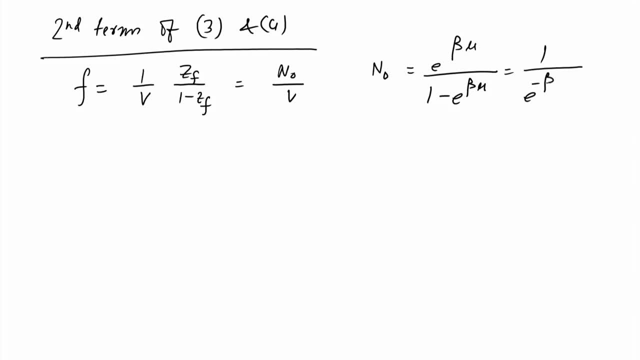 beta mu, which is nothing but equal to exponential minus beta mu minus 1.. So this is the N 0 by V. that is the second term in equation four. So this is four now, when your Z F is much smaller than 1. now Z F is actually between: 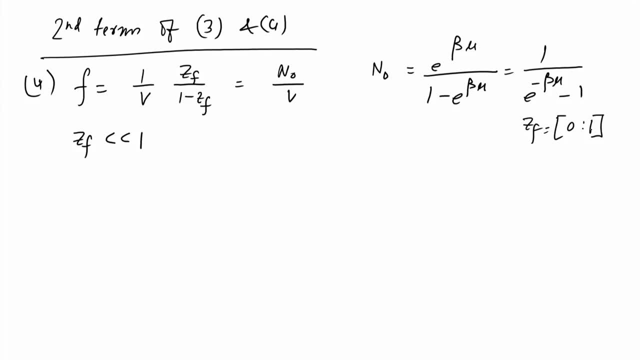 0, and So it can take a maximum value 1 and it can take a minimum value 0. So if Z, f is close to 0, that is smaller, much smaller than 1. then we have. So this corresponds to very large. 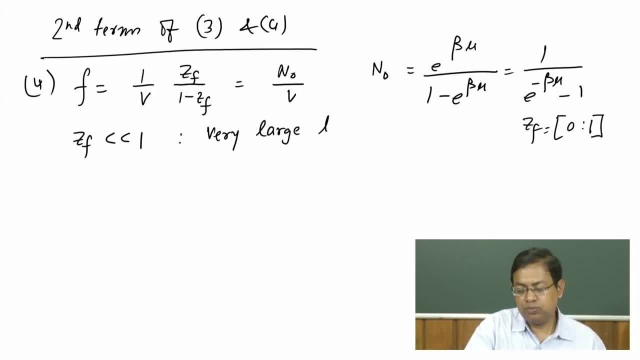 temperature, and if it talks about very large temperature, then you have the number of particles is very low, because this f is equal to f is very small and So N 0 is very small and of course that corresponds to no Bose Einstein condensation, because you have a classical 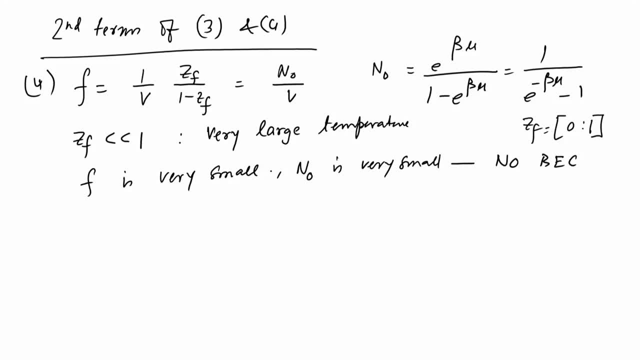 physics that is taking over. So thermal effects, would you know, drive all the particles away. Now you try to understand that as you reduce the temperature, N 0 increases. So at very low temperature, N 0 is very high, and So as Z, f goes to 0.. 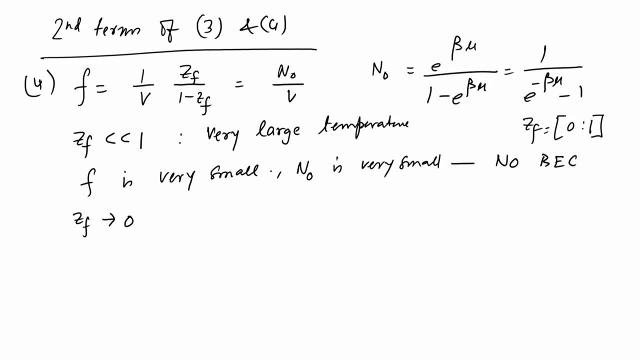 So that is So. mu is actually a chemical potential which is negative. So if Z f goes to 0, then N 0 by V is significantly large. In fact it is so large that your N equal to N e, x plus N 0, somehow, if you can show. 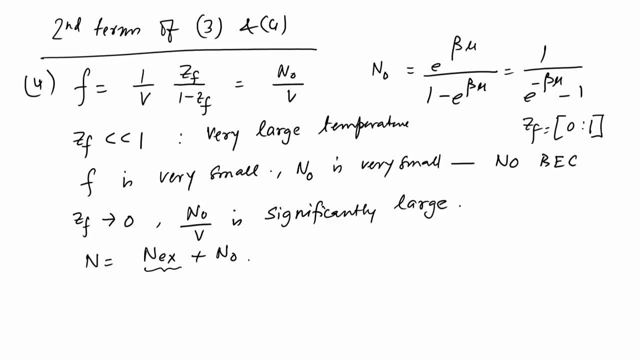 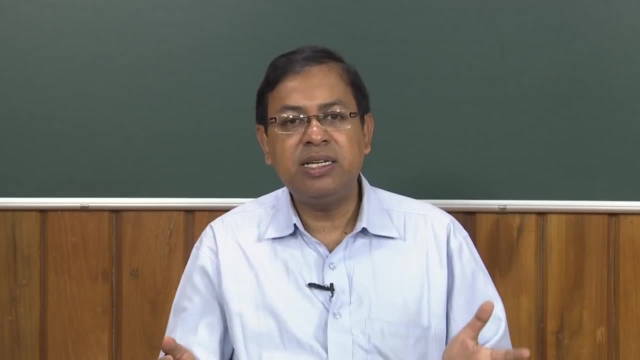 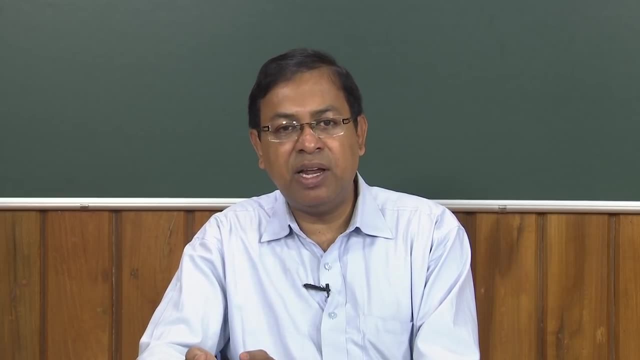 that your N, e, x is equal to a finite number, Then since N 0 is infinitely large. so if your N is infinite, or rather very large, then all the particles will go to the ground state because it has infinite occupancy, whereas a very smaller number of particles would actually. 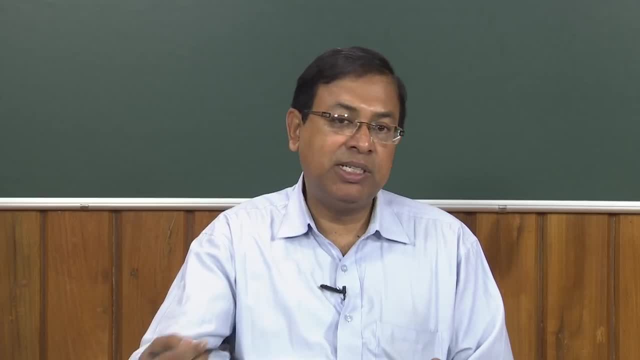 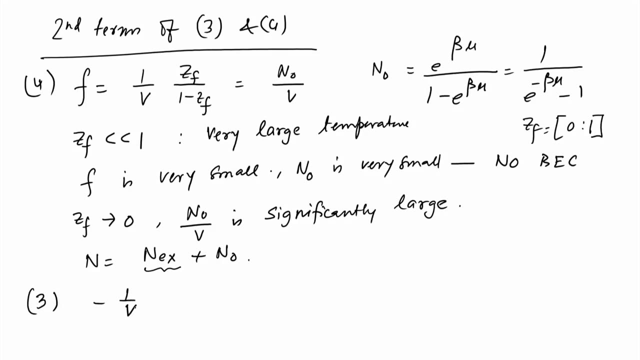 go to the, the excited states, because it has limited occupancy. Now, if you look at through 3, then you will see that this is equal to the 0, epsilon equal to 0. contribution is equal to this and this tells that for Z, f much smaller, then this is equal to negligible. So this 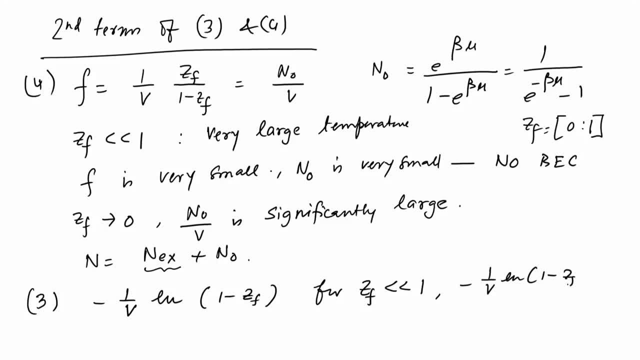 minus 1 over V log of this thing is very small, that of course we know that the pressure due to the all the particles that would go to the ground state is very small because there is no, almost no particles at large temperatures. This is the limit for large temperature. However, 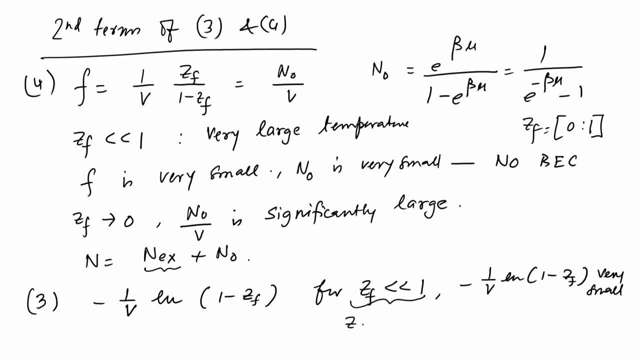 if you go to the other limit, that is Z f going to 1. I am sorry Z f should go to 1 here, not 0. So Z f is 1.. So if Z f goes to 1, so this is for Z f. 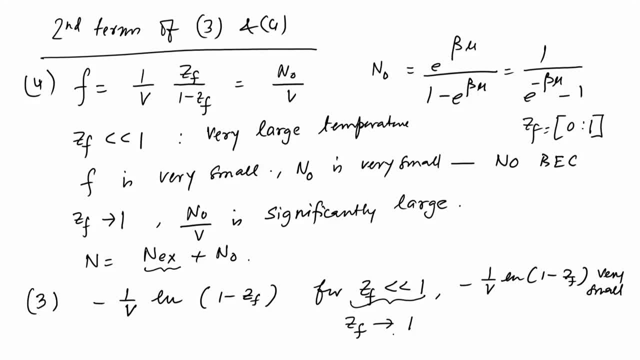 going to 1.. So Z F going to 1.. However, this thing would take a form which looks like 1 over V. log of N naught. Now, N naught could be large, but log of that would be, you know. 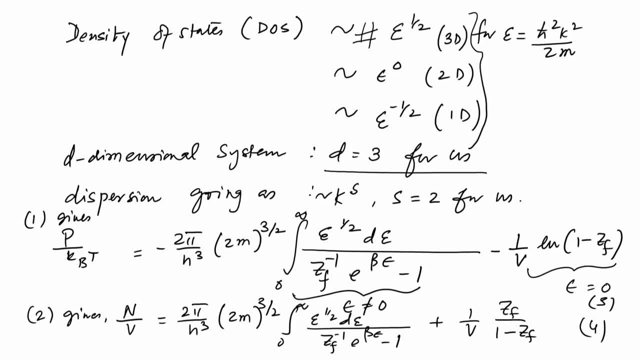 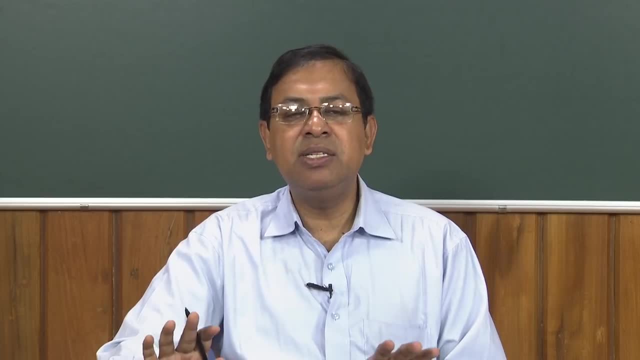 still small. So the second term in equation 3 can still be neglected, even if at low temperature that is Z F going to 1 or the fugacity going to 1.. However, that cannot be neglected in equation 4.. This is the main central message of this discussion: that even the pressure 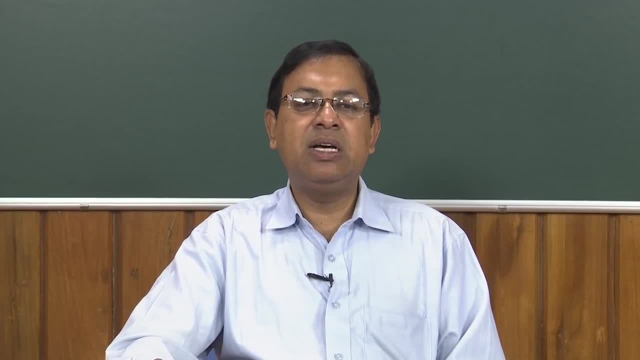 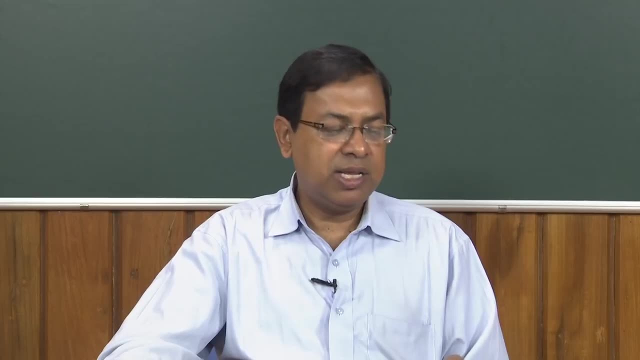 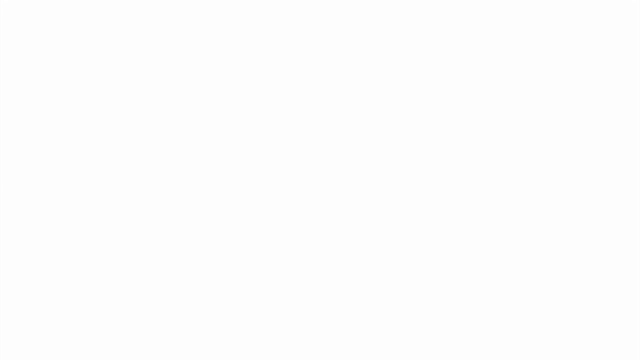 contribution from all the particles in the ground state of the system could be infinitesimally small. However, the number of the number, density, is significant. So now we will write this Then. so basically, my our 3 becomes its P over k. T is equal to minus 2 pi over h cube. 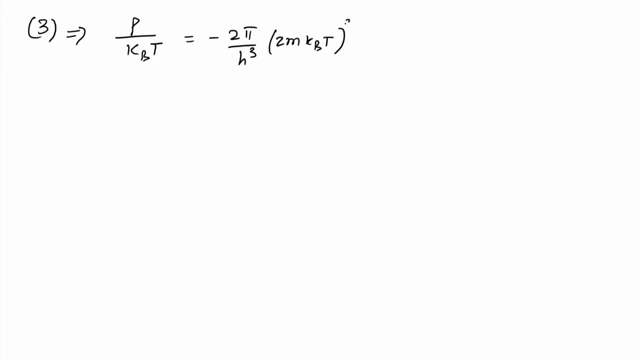 2 m k, T whole to the power 3 by 2 and 0 to infinity, x to the power half. So it is log minus Z, F, exponential, minus x, d, x, where x equal to exponential minus, sorry, x equal to beta E. that is the thing. 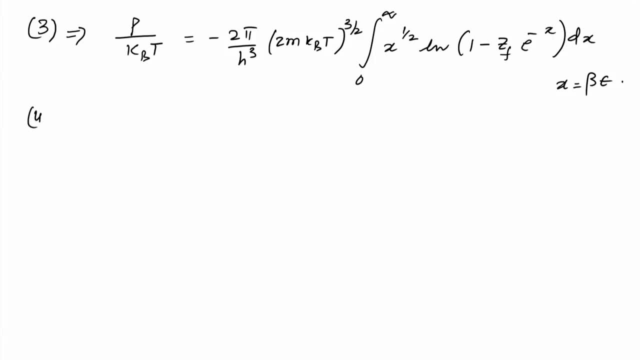 And so beta has come out and the 4 gives- let us call this as maybe 5- and 4 gives N minus N, 0 by V, Which is N e x by V e x. N e x is the occupancy or the number of particles in the excited. 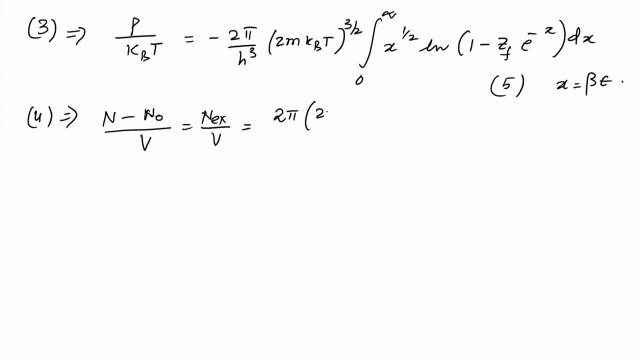 states, and this is equal to 2, pi, 2, m, k, T by h cube and this is equal to: So this is 3 by 2 and this is equal to x to the power, half d, x, Z, F. Now these are called as the Bose, Einstein Integral and G N of Z. So this, these are: 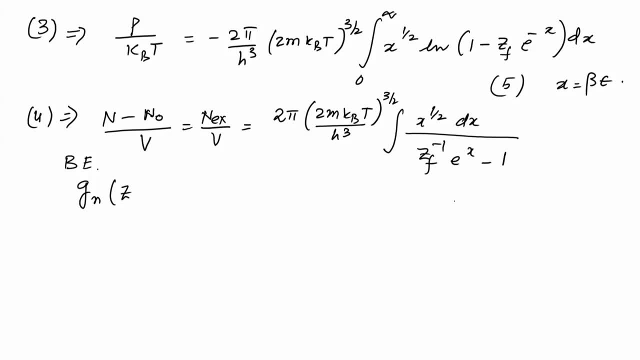 Bose, Einstein, Integral in short, called as Be Integral. and this Be Integral takes a form: it is equal to 1 minus gamma, N, x to the power, N minus 1.. n minus 1. you can write it as Z, f, and this is equal to d x divided by 0 to infinity. and. 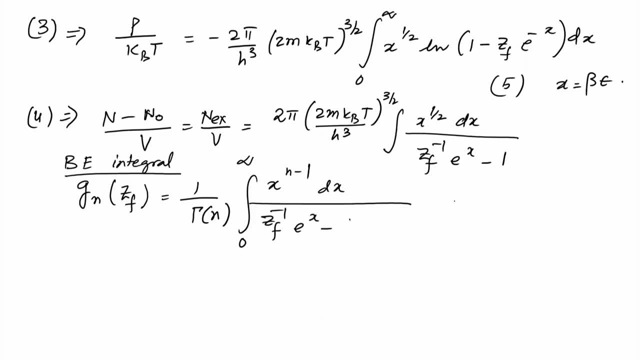 it is equal to Z, f inverse exponential x minus 1.. So these integrals look very similar to that, excepting for its n equal to, say, 3 by 2, and so on. So, and this is equal to, it can be shown this. I leave it to you, it is a matter of you know doing a partial integral integration. 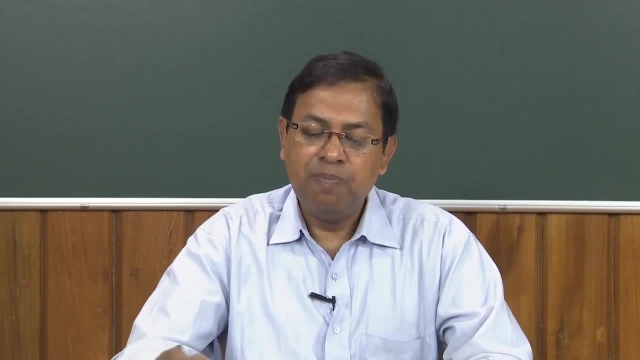 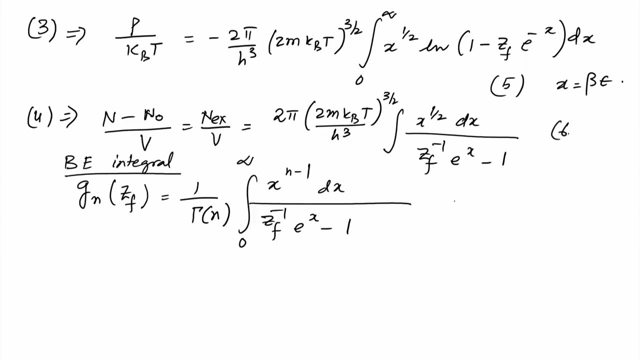 sorry- integration by parts of this integral and express it in the form of this, and finally what one gets is: So let us call this as 6.. So 5 becomes equal to p over k. t is equal to 1 over lambda cube. 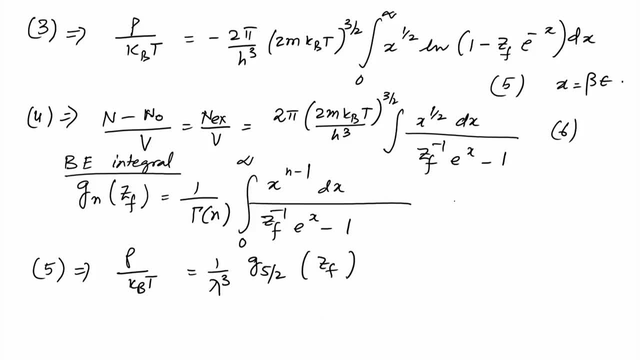 And G, 5 by 2, Z, f. we are less interested in this formula, though it is important nevertheless. However, we are interested in this formula then, one that we are going to write later. So let us call this as 7, and this is equal to n, e, x by v, which is equal to 1 by lambda. 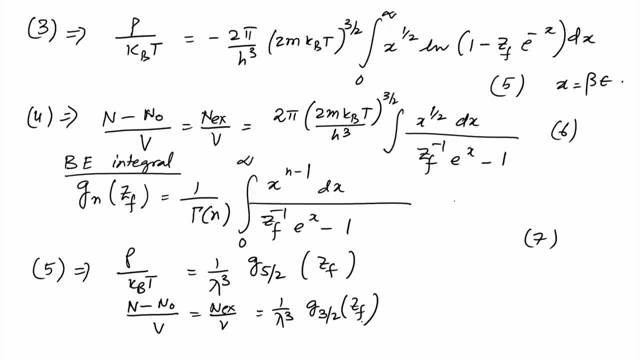 cube G 3 by 2, Z, f. that is the second equation, that is equation 6.. So 6 yield this. So now our. the number of particles, which is what we wanted in the excited states, is given by some quantity, which is this: well, lambda is equal to root over h over h, divided by: 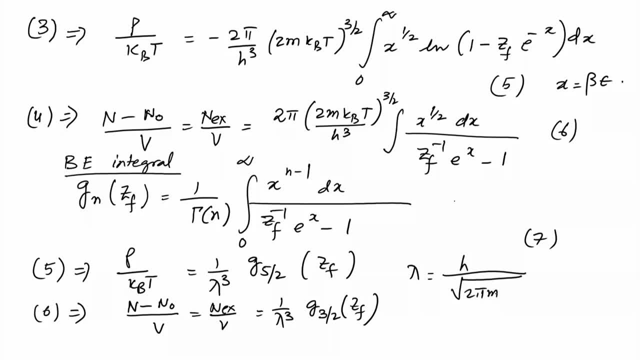 root over 2 pi m 2 m kt. Sorry, not 2 pi m 2 m kt. It is called as 2m by 2 m kt, So this is 2m by 2 m kt. Sorry, 2 m. 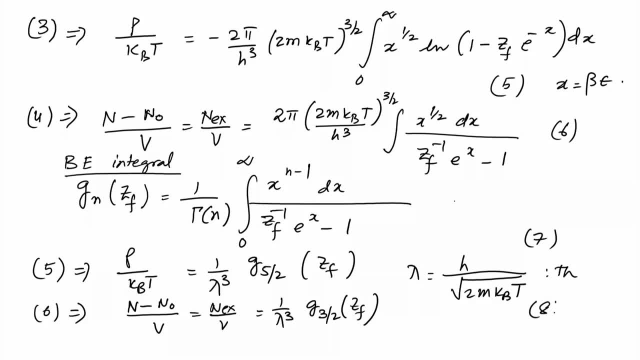 2m by 2pm, by 2pm. So here I did not include the number of particles here. So 2m by 2pm called as a thermal de Broglie wavelength. So this is equation 8: thermal de Broglie. 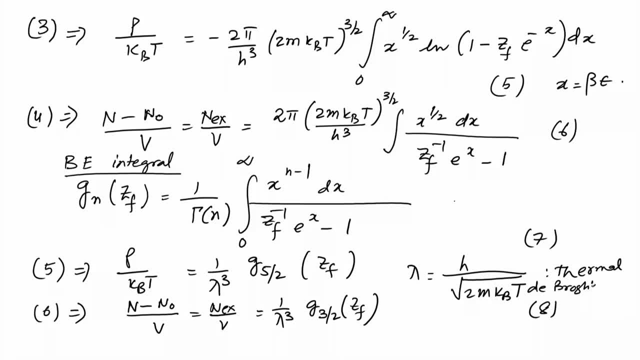 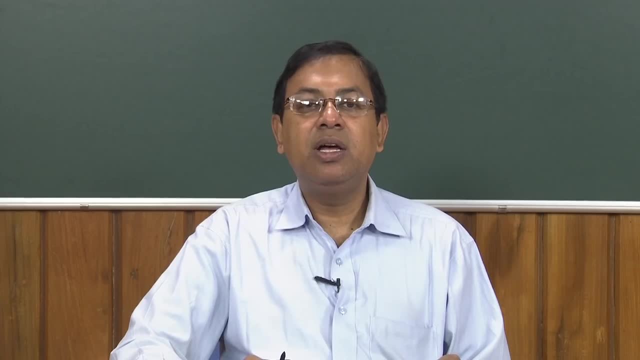 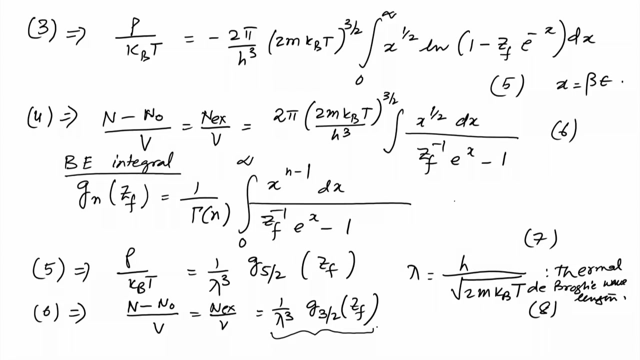 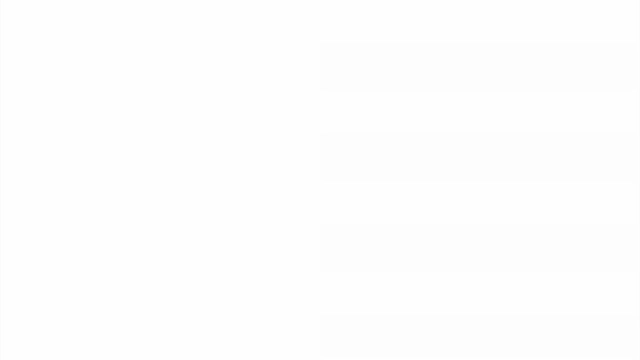 wavelength. Now we are almost done. we have obtained an equation for the number of particles in the excited states. If this quantity is finite- it is not infinitely large, which would depend upon certain criteria- then we are done. We would again leave this thing and show that your G n, Z, f is equal to sum over L equal. 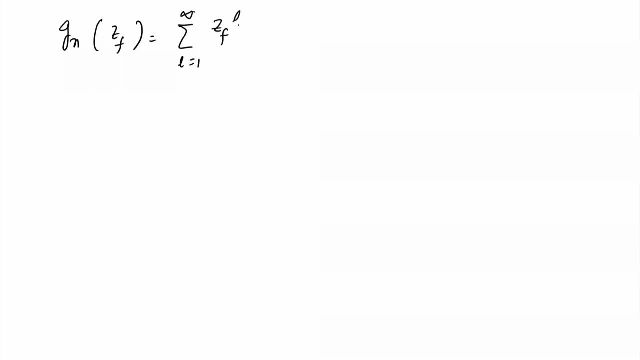 to 1 to infinity. It is a Z f to the power L, L to the power n, which is equal to Z f plus Z f square by 2 to the power n, plus Z f cube by 3 to the power n, and so on. Now for small. 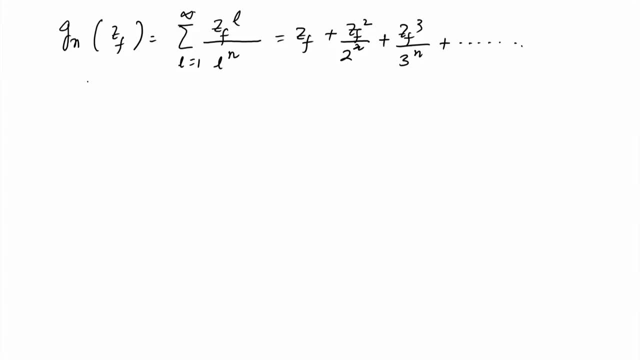 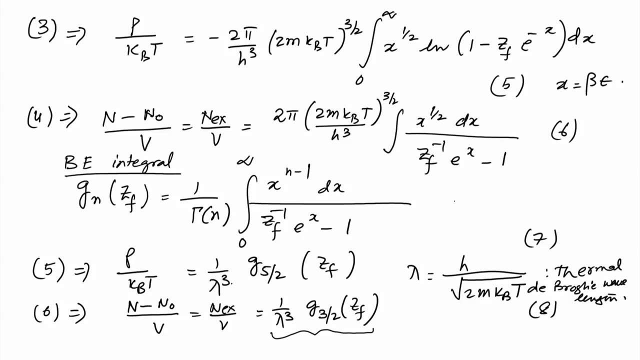 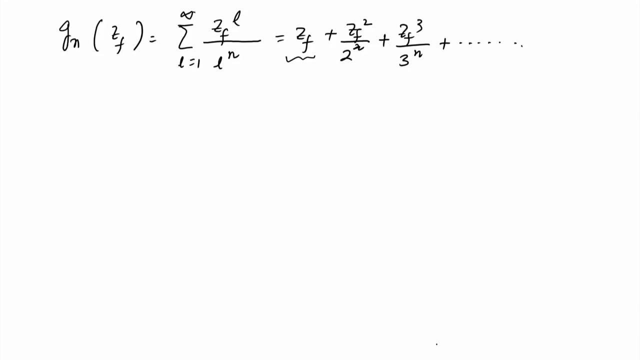 Z f. that is Z f much smaller than 1, the classical limit. you can be satisfied with Z f, ok. So if you put that equal to Z f then of course that becomes will depend on the excited state occupancy is. you know is goes as exponential beta mu. However at low temperature, that is when Z 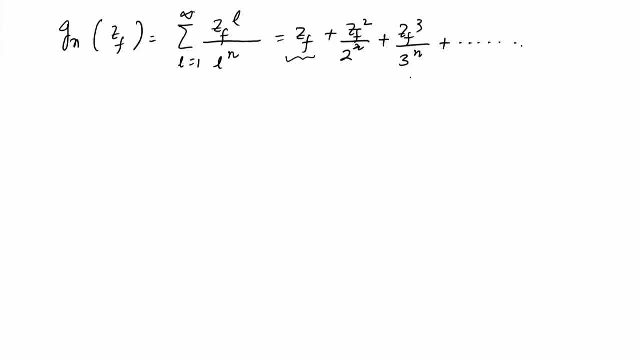 f goes to in the limit goes to 1. you have to take all of these terms into consideration and cannot stop at a finite terms, but fortunately this is equal to for G 3 by 2, Z f, G 3 by 2 and Z f equal to 1, which is of interest to us, this is interesting to us and this it is. 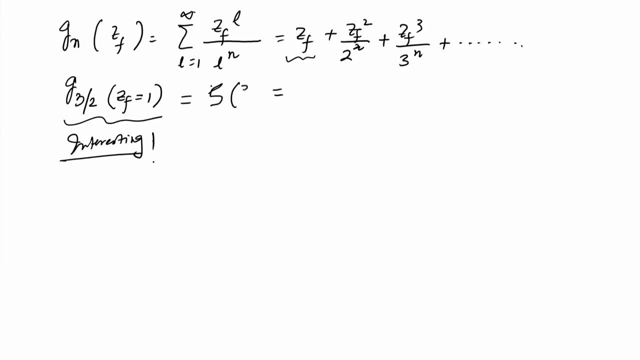 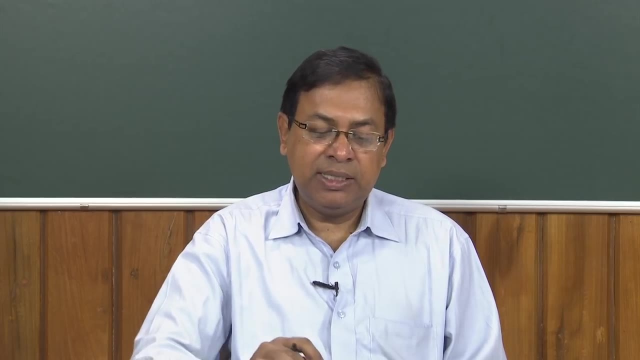 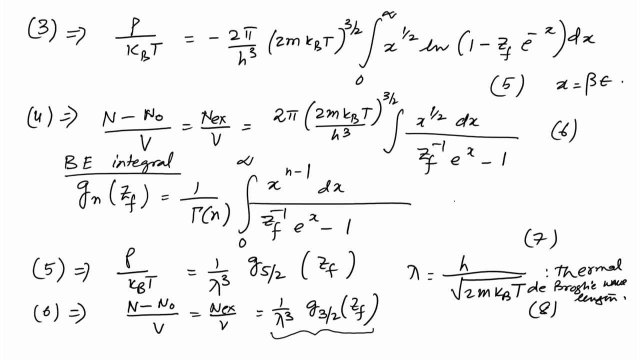 equal to a Riemann zeta function which is 3 by 2, which has a value 2.612.. So this is a finite value. this is what we were hinting at time and again: that the excited state occupies which are coming out from this equation number 8 has an. the excited state occupancy has a. 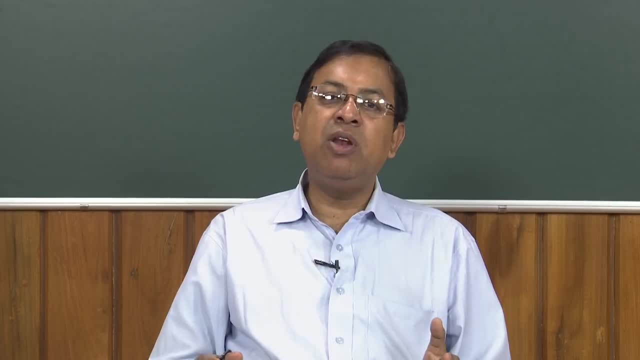 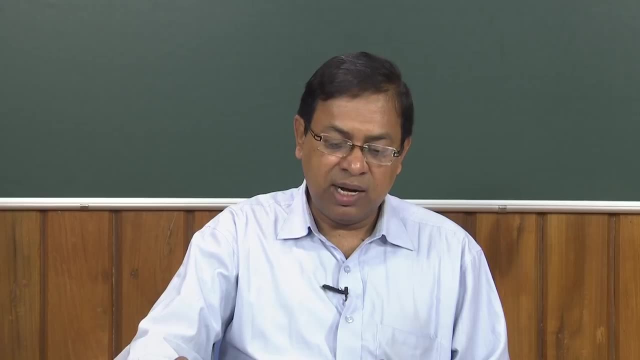 finite value. So if there are more number of particles, they will all go to the ground state. if there are macroscopically large number of particles, they would all go to the ground state. and this is what the condensation So, n greater than you know, a, V, t to the power. 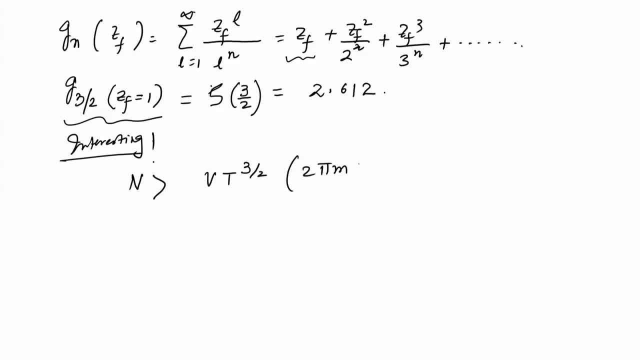 3 by 2 and 2 pi m k divided by 2.. 3 by 2, h, cube, etcetera, it becomes equal to a 3 by 2, and this xi is. this is not the way to write. it is like this it is called as the Riemann zeta function. So the Bose Einstein. 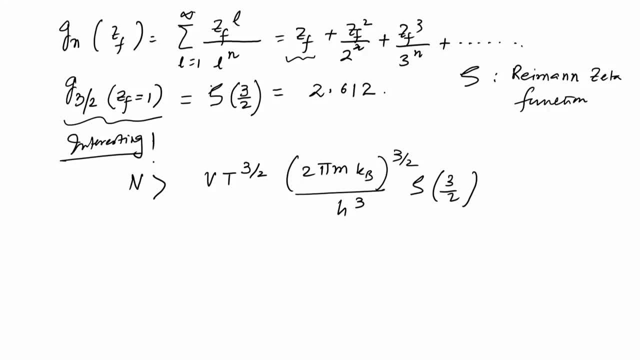 integral is related to the Riemann zeta function. when you take this entire sum, the entire sum has a closed form. So this is called as Riemann zeta function and for an argument equal to 3 by 2, it has a value equal to 2.612.. So if n is greater than this, n is the total number of particles. 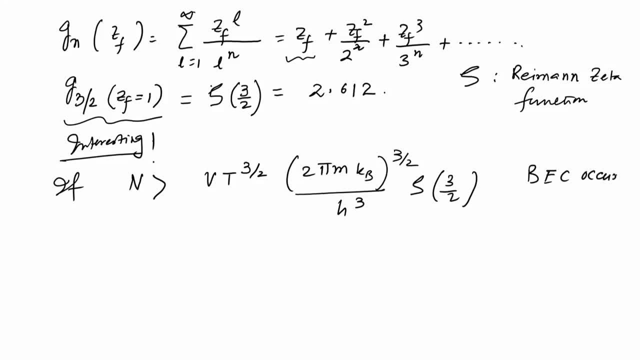 then BEC occurs. and for the BEC to occur, the critical condition is that your n by V has to be equal to some T c 3 by 2. it will happen at that value. So this is equal to a k 3 by 2 and by h cube, and this value, which is equal to 2.612. 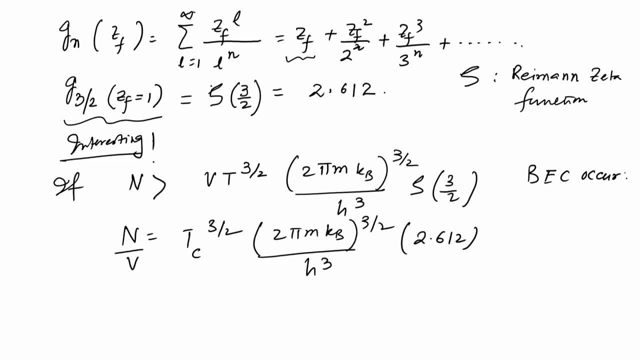 So if you put everything there, then what we get is that a, T, c has an expression which is equal to h square by 2 pi mk, and it is equal to n by V And it is equal to 3 by 2.. 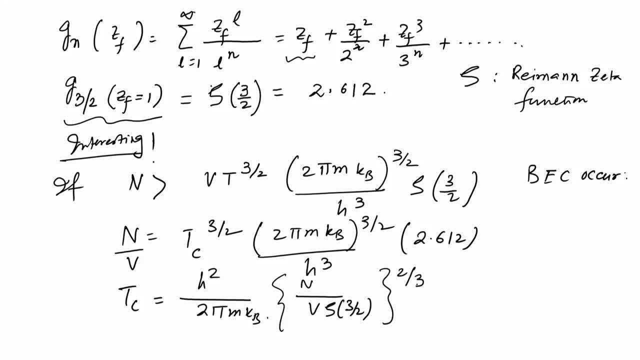 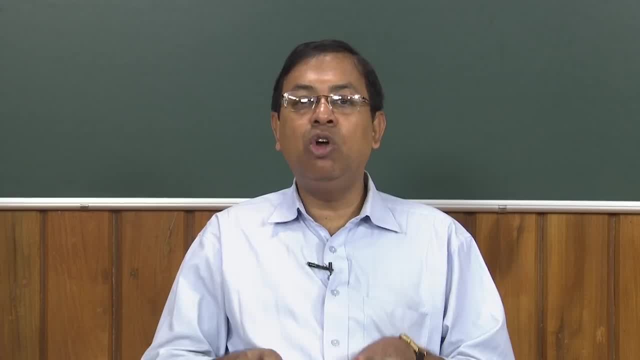 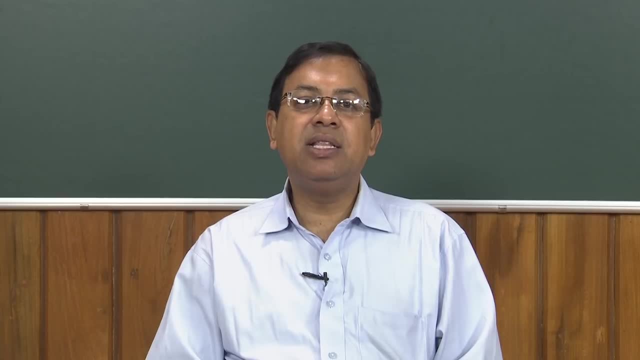 2 and it is equal to a 2 by 3.. So this is the expression for T c, which means the temperature. if it is lowered below this, then all the particles will go to the ground state and the excited state, because the excited states have a finite occupancy. they will avoid the excited states. 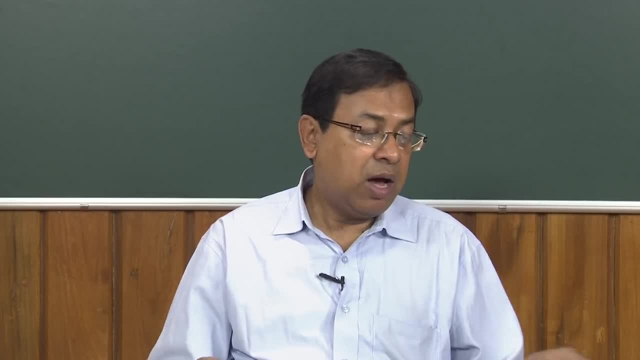 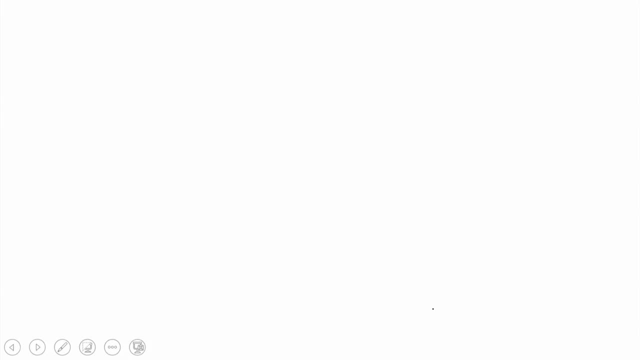 and go to the ground state because the temperature is also very slow. Now, this we will just do it for helium 4 which, as we said, that is not a prototype case for Bose-Einstein condensation, but still, if you take this, values is 10 to the power minus. 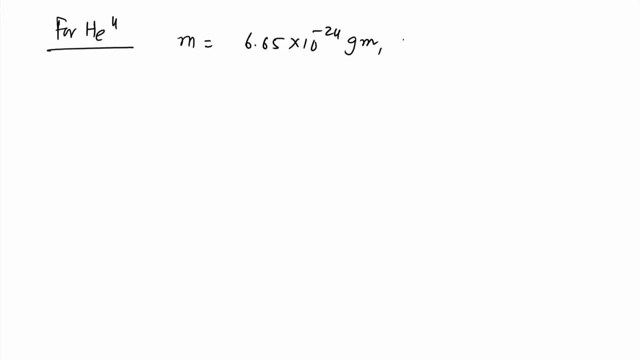 24 gram, and So the density or the inverse density, So inverse density, or which is called as a specific volume, V by n, equal to 227.6 centimeter cube by per mole. then if you put all these things, T, c comes out to be equal to 3.13 Kelvin. 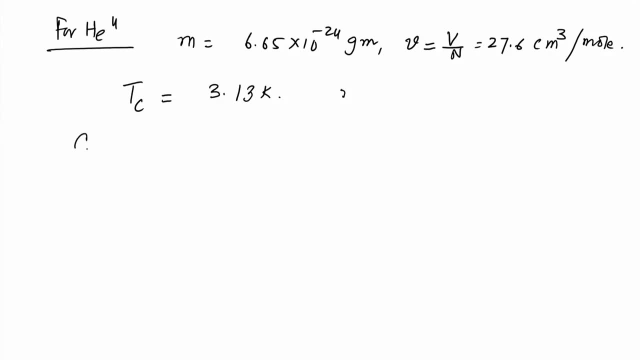 and 13 Kelvin, And this is close to the observed lambda point transition Of helium: liquid helium, liquid helium, which is equal to 2.17 Kelvin. So there was a initially a misconception that the liquefaction of helium is actually, or rather the lambda point transition. 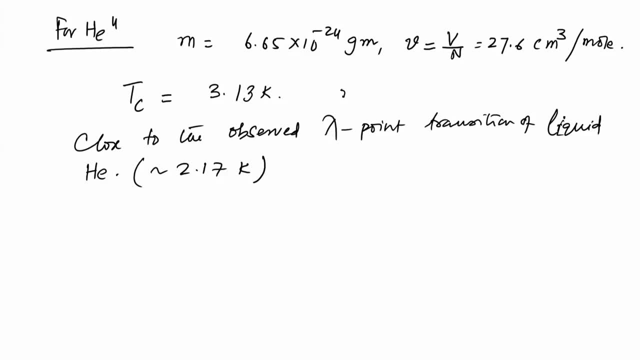 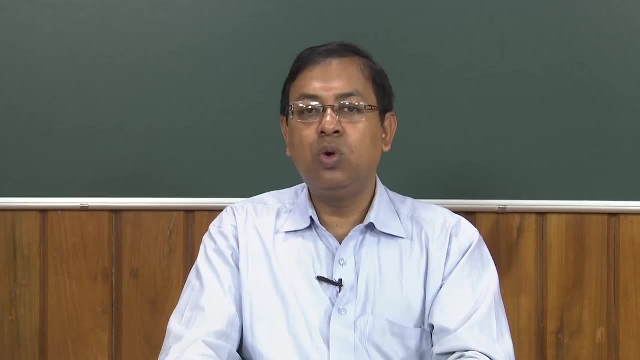 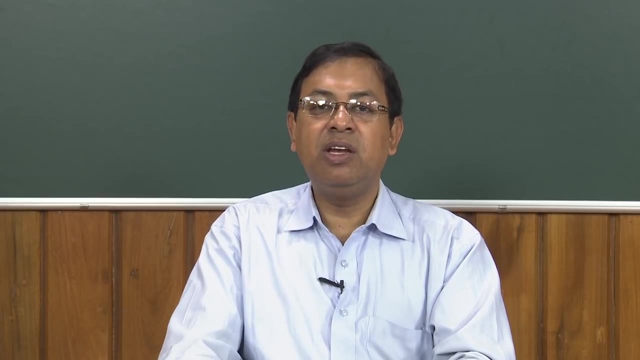 in helium is actually a B E C transition. We will not elaborate on that, but what we have gotten is a condition for the Bose-Einstein condensation. Also, we have explained various steps that are associated with the cooling process And finally, when the cooling happens, the whole atom, either the 10 to the power 6 atoms number. 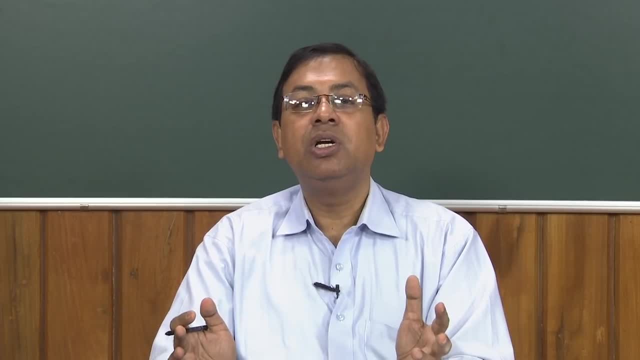 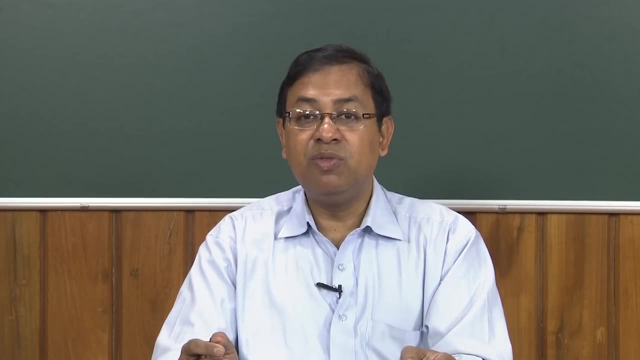 of atoms. they form a structure which has very low temperature, which is like 10 to the power, minus 6 to minus 7 Kelvin, which is like a less than Nano Kelvin about micro Kelvin temperature, which is the probably the coldest temperature in the universe. 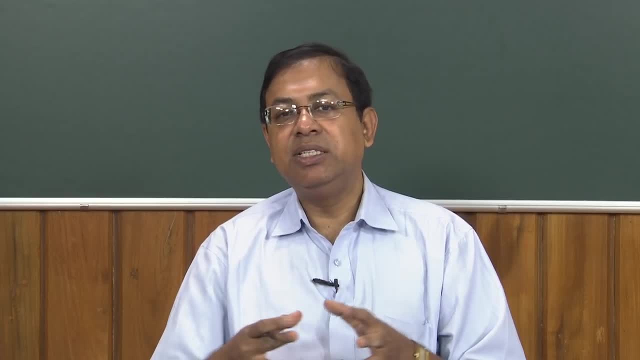 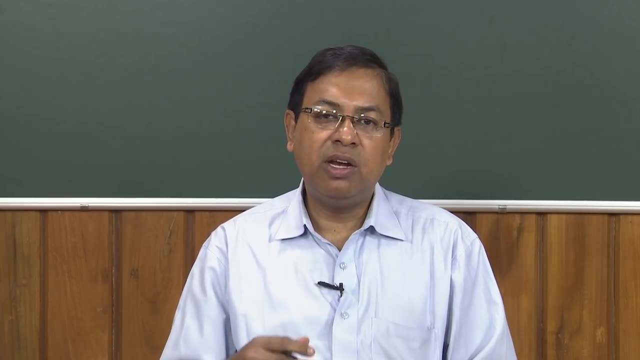 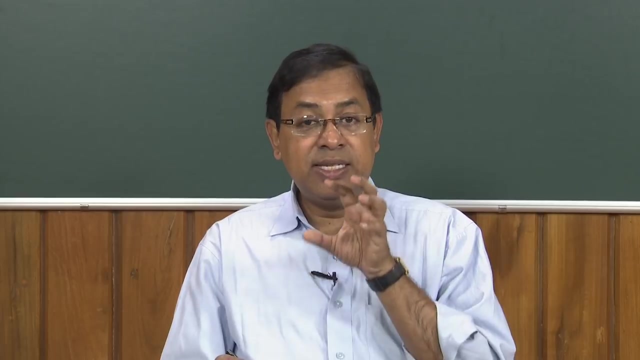 And they are imaged, as I said that, releasing the traps and letting them fly apart. So when they fly, they are imaged and they are finally, Fourier, transformed into k-space. to see there is a macroscopic accumulation of particles in the k-space. So this is a k-space. 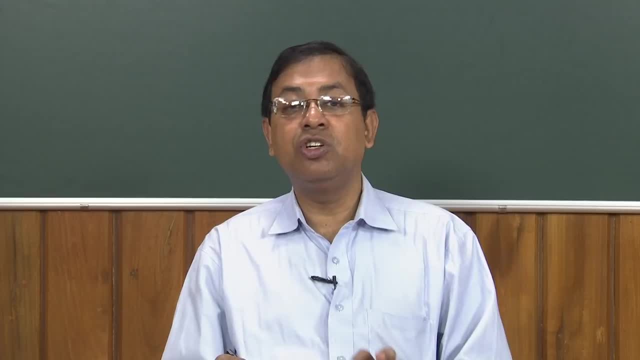 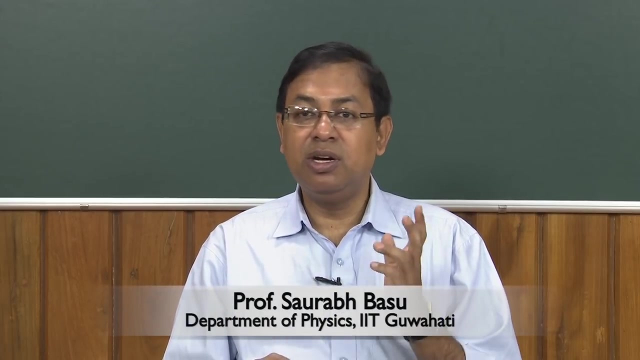 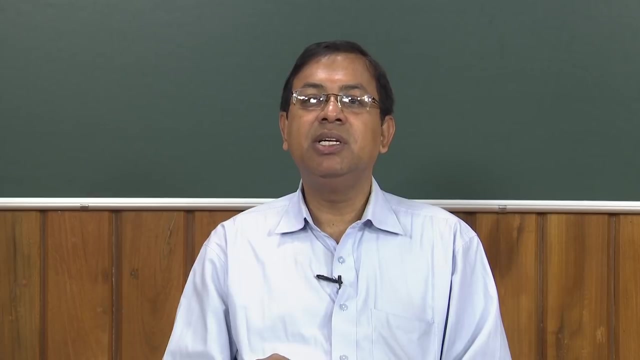 phenomena. it is a real momentum space accumulation of particles. the BEC is a example of that, And so this the credit goes to Bose and Einstein, who have proposed this in 1924, nearly 100 years from now. 100 years earlier, However, as I said, the realization had take place very 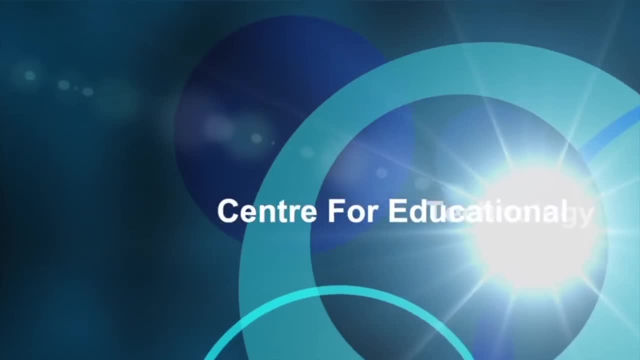 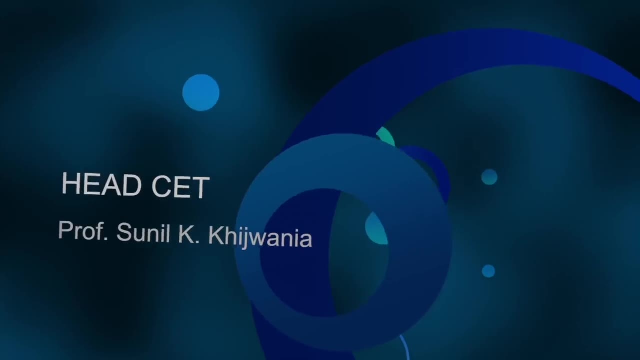 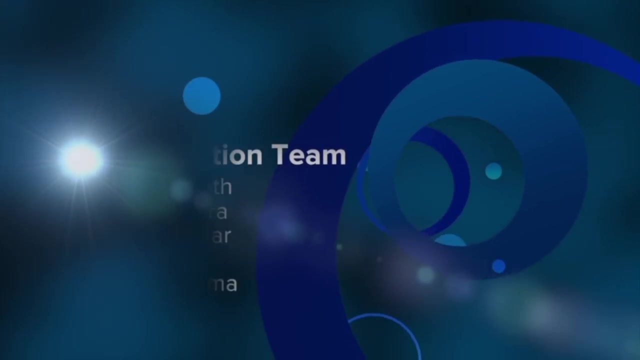 large number of years. Thank you very much.